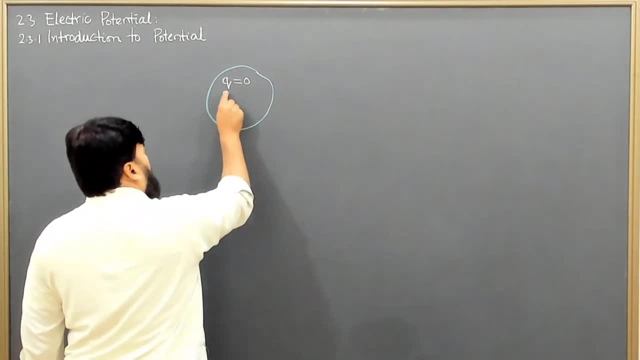 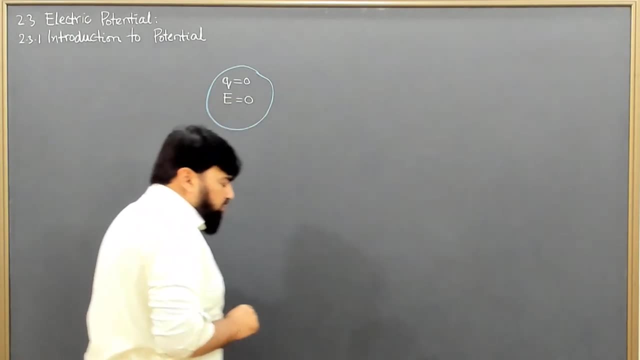 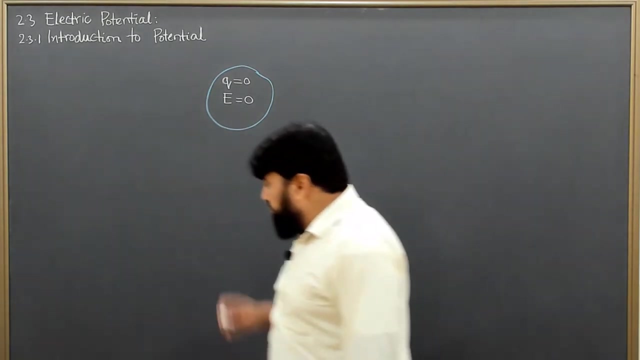 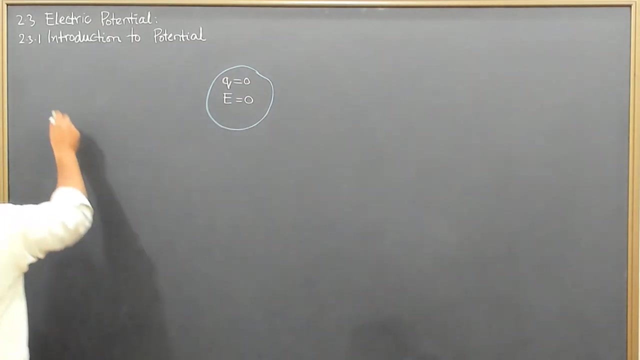 the source charge is equal to zero, then this will tell us from Coulomb's law we came to know about this thing: the electric field will be zero and that region is the source charges are equal to zero. Now if, for example, we are having two positive charges, like we are having a positive charge here and a positive charge here, and both are of positive charges- 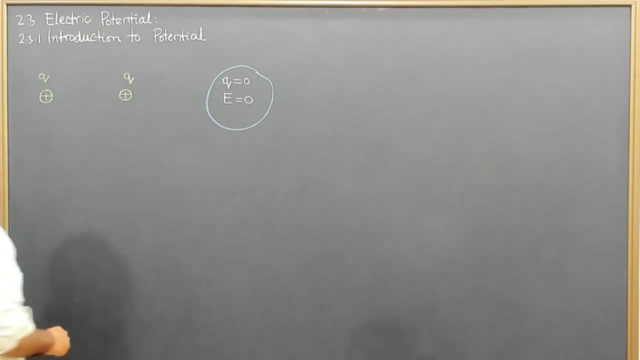 the same magnitude, Q and Q. Then what is the electric field at the center? Now, the field at the center is E equal to 0.. The electric field at the center is E equal to 0.. Now let us look here and here These are two different scenarios, Like, for example, we are having this region here. 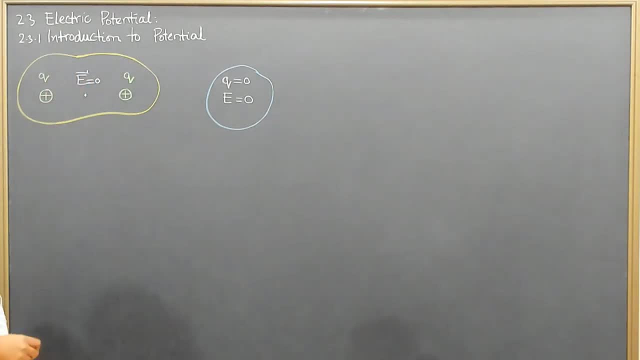 any arbitrary region in which we are having this situation. Now look here. Here the electric field is 0 by magnitude. Like: the magnitude is such that the electric field is equal to 0. Now let us look here and here. These are two different scenarios- Like, for example, 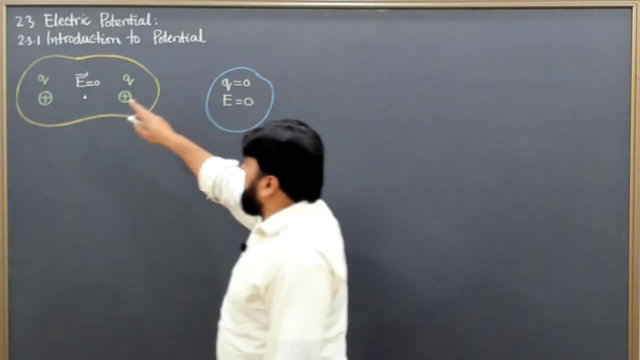 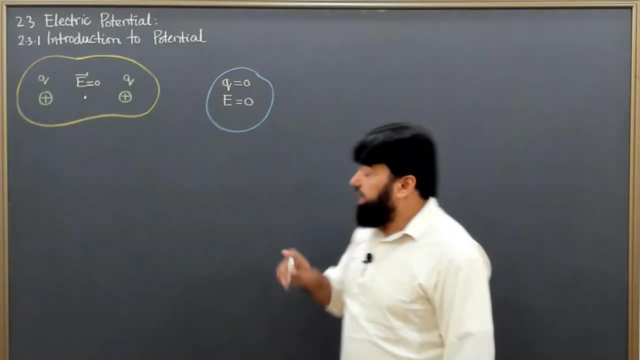 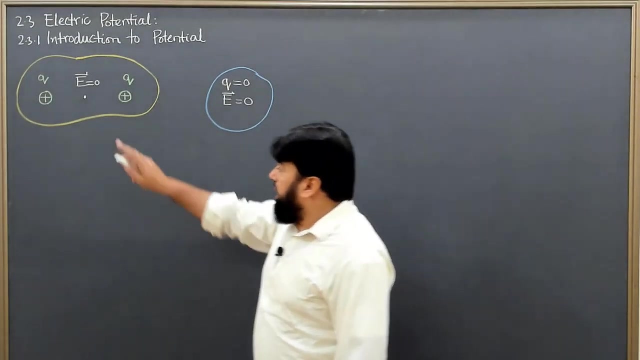 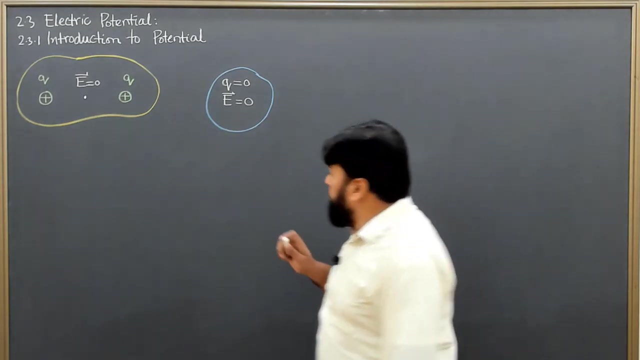 to 0.. And here the electric field is 0 by magnitude, but not due to the source charges. Here the electric field is 0 because there are no source charges. Here are the source charges, but the electric field is 0. Now, these two things are 0. This, we say that this is due to the source. 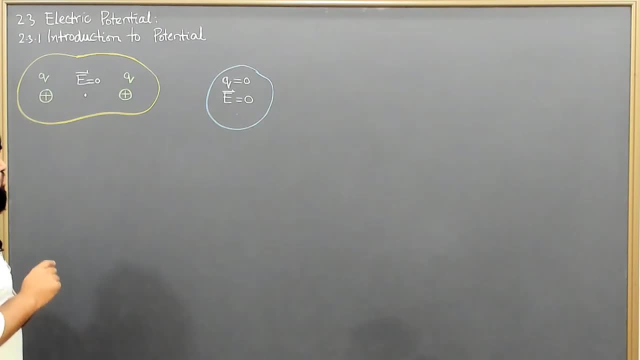 and this is due to the geometry. So to E equal to 0, how we will tell the mathematics that this E equal to 0 is different from this E equal to 0. And there comes the need that this one is coming out to be 0 due to the reason. 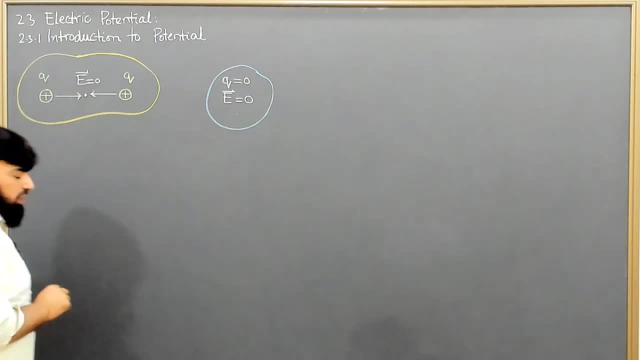 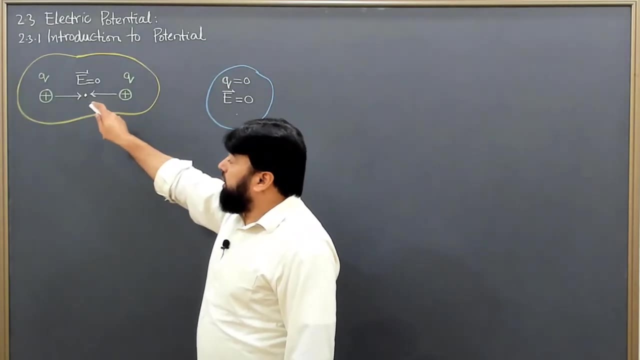 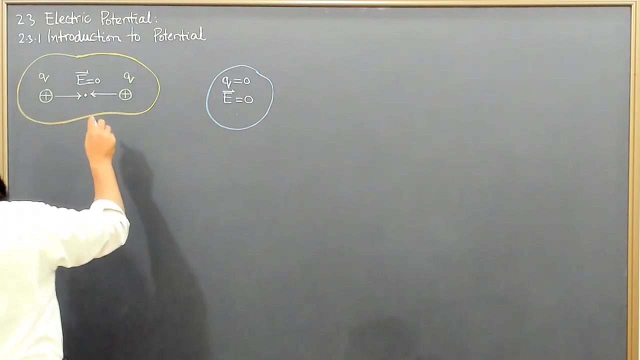 that the two electric fields are cancelling each other due to their vectorian nature. So the concept of electric potential comes here, that we need something that depends on, not depend on. the vector form is not supposed to be vector in nature, but to be a scalar, And here V will not be equal to 0. But here V is equal to 0 as well. 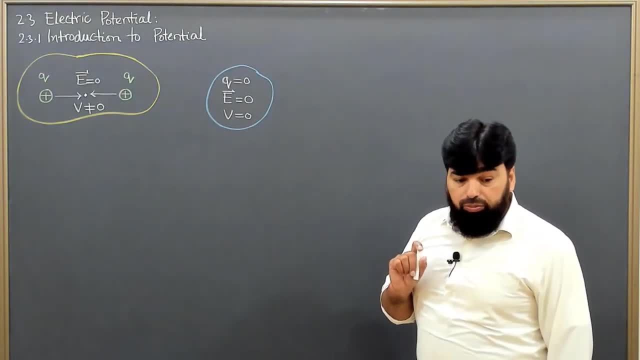 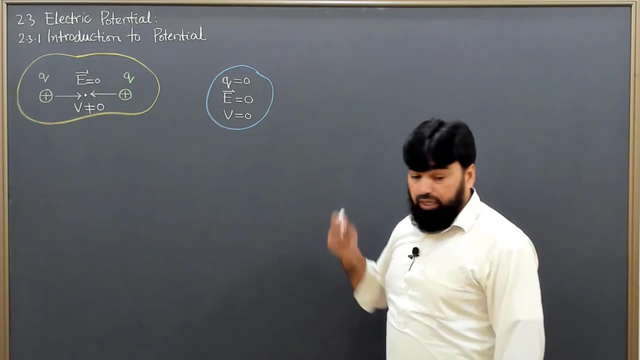 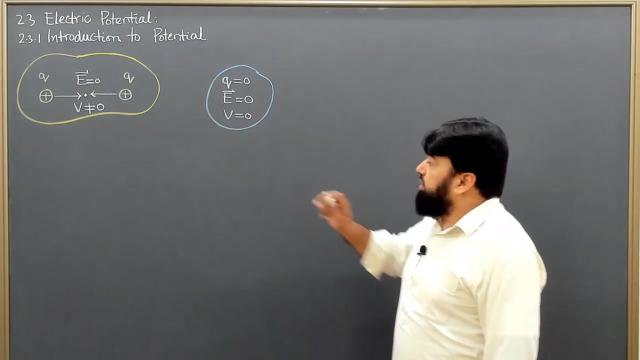 So the vectorian nature was giving us a problem there and it was giving us 0. Then we got rid of this thing by introducing its scalar counterpart, And that's why we will. now we can easily differentiate that here it's a different. 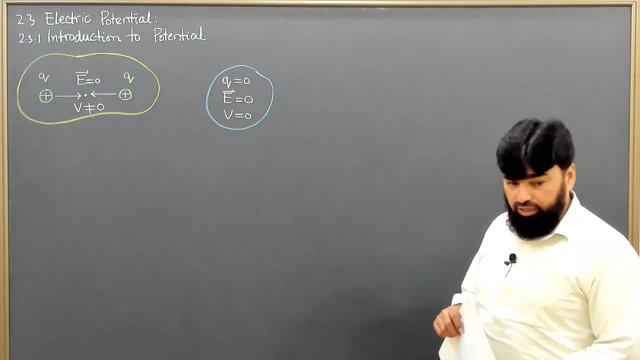 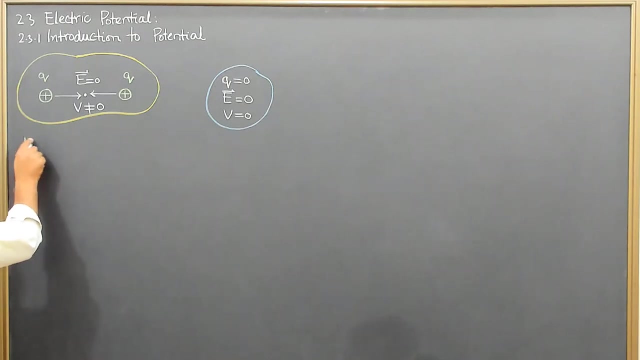 scenario, and over there it's a different scenario And there is a need of defining electric potential. Now we know that when we are talking about electric potential, we are talking about electric potential. So when we talk of electric field, then electric field is not an ordinary vector. 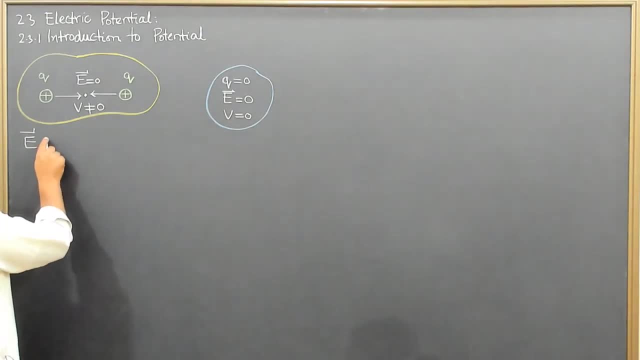 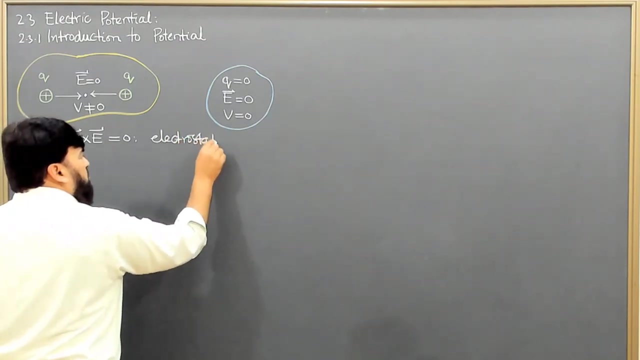 an ordinary function, but it's a special kind of function, such that its cross is del cross. its curl will always be equal to 0 as long as we are in the regime of electrostatics. I am not talking of the electrodynamics, because all there. 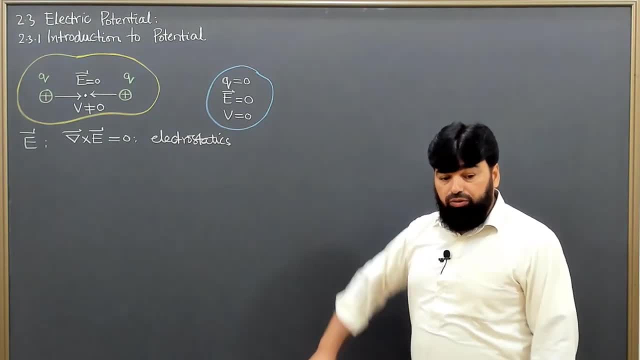 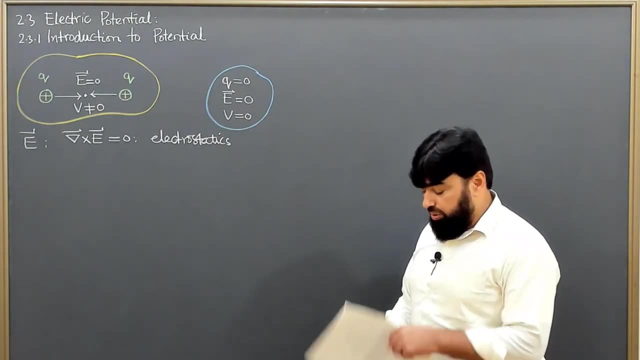 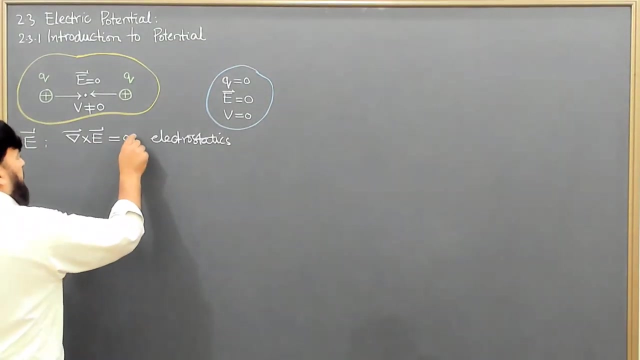 the curl of E is non-0, as we know, in Faraday's law of electromagnetic induction, The paradise, love del cross. equal minus curly P by curly T, So here, as long as we are here, then V in electrostatics, So we will have the curl of E. 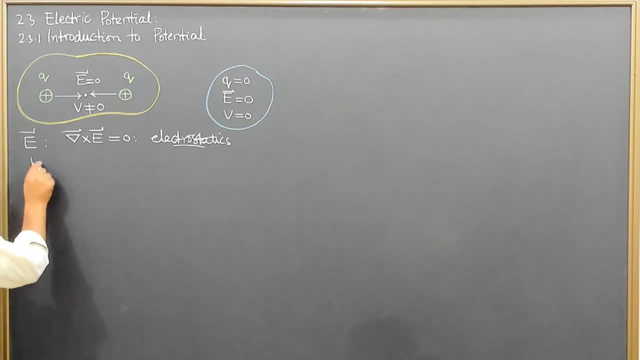 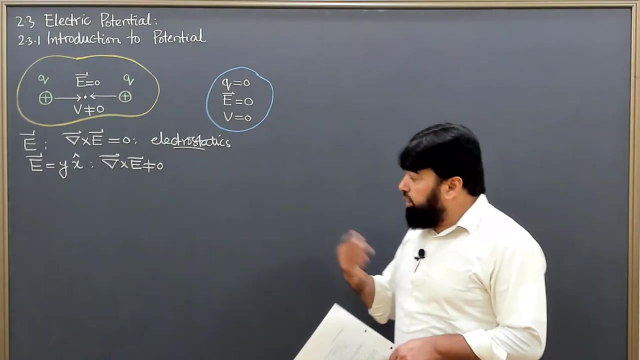 equal to 0 means it is not possible to have electric field like this, for example like y in the x unit vector, Because for this kind of vector del cross, e is non-zero. You can check this thing. This is non-zero. So there is no such charges or combination of charges. 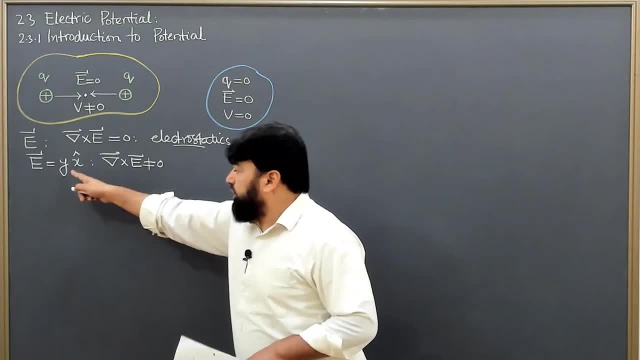 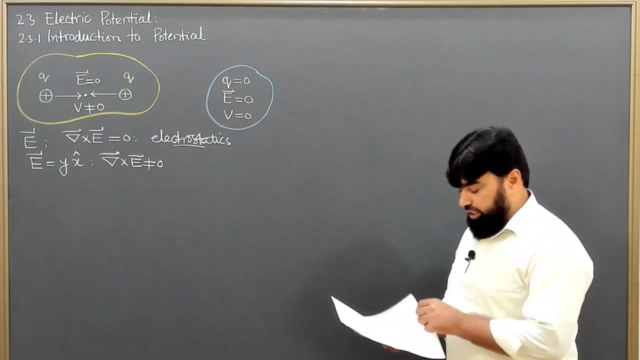 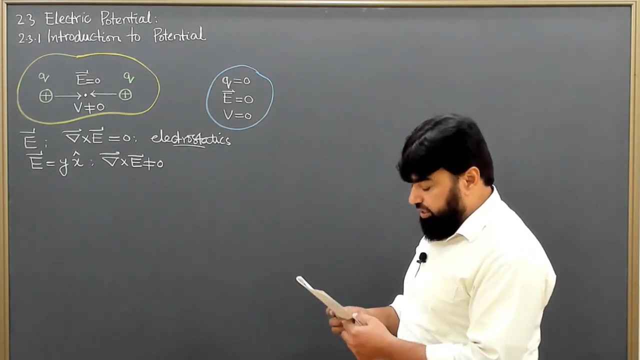 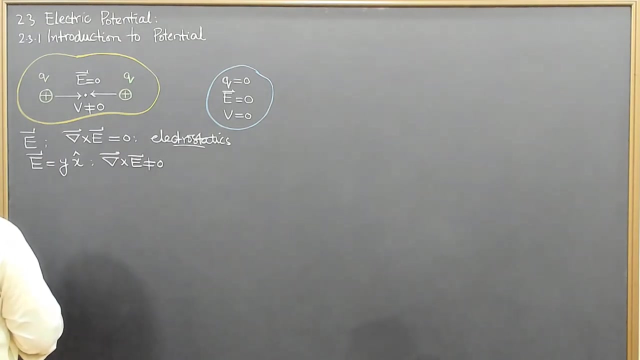 which can produce such a field. So it's a special kind of a function or a field which has its curl equal to 0. And now we define the electric field. that this thing we came to know from here, that when del cross e is equal to 0, then it's not possible to have 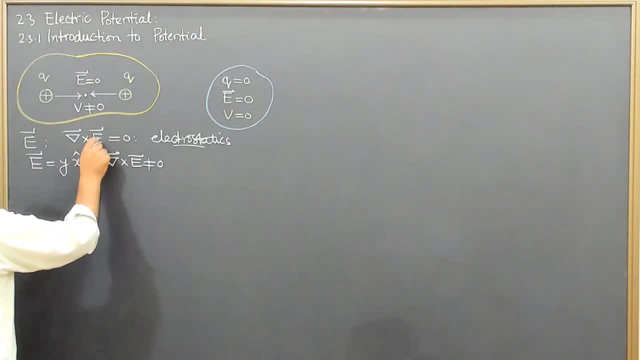 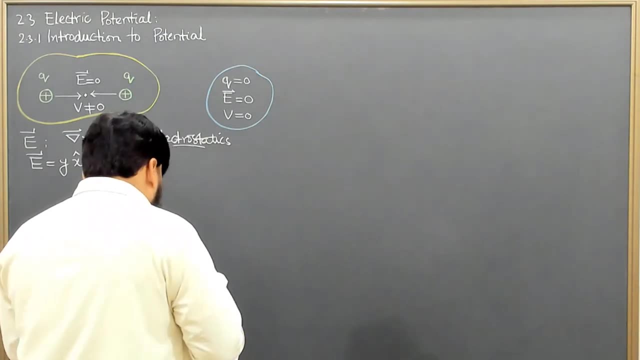 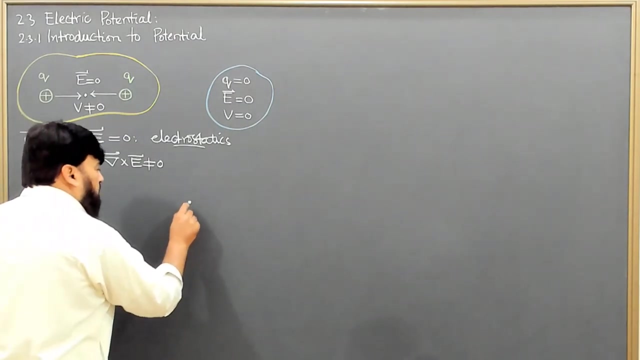 electric field. So it demands that this e is the result of the gradient, of something which we have studied in chapter first. So I can define that if I'm like. for example, the endpoint does matter when the closed loop integral of this thing is equal to 0, like. 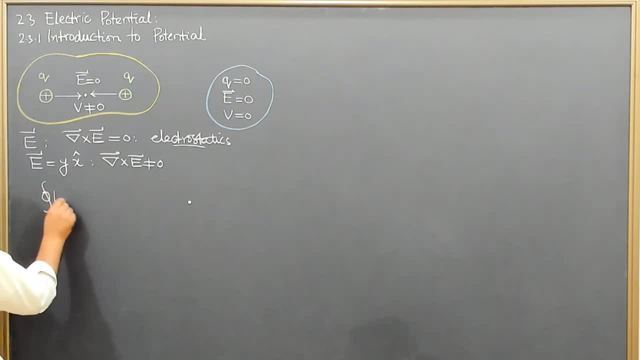 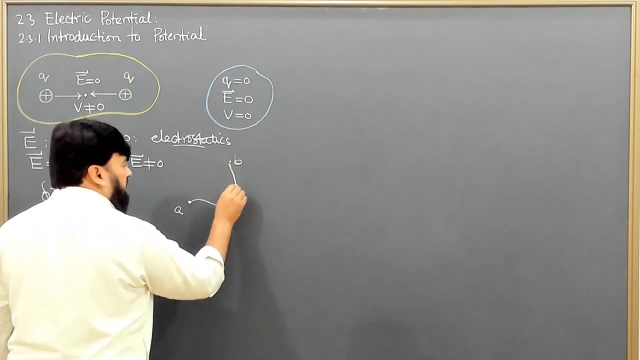 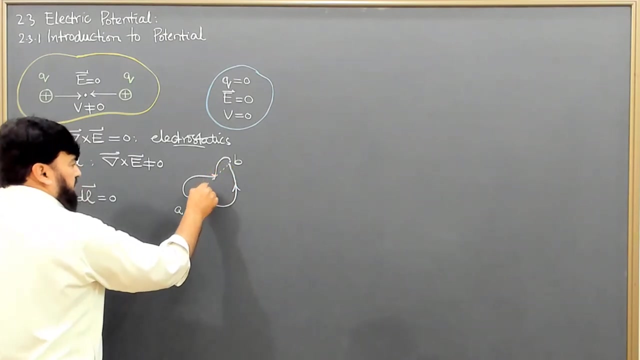 the earlier we did this thing, that e dot, dl Is equal to 0 around a closed path. So it doesn't matter, while moving from A to point B you go this path or you go this path, It doesn't matter. Only the endpoints does matter. 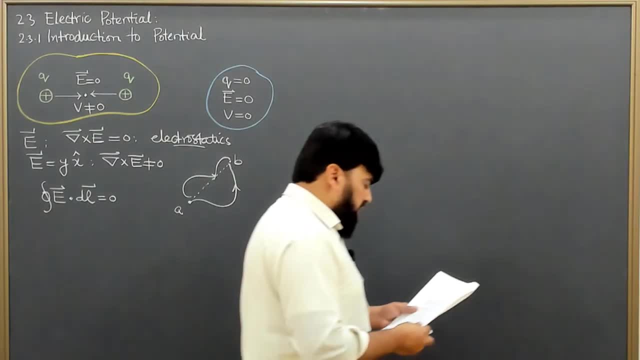 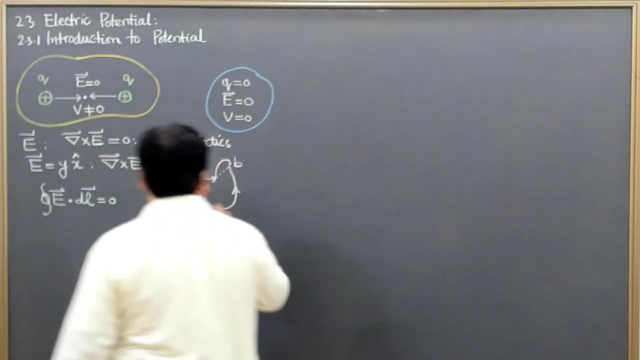 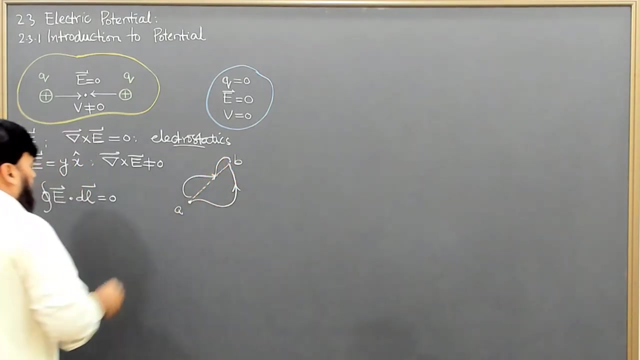 and such a field we call a conservative field. And if it would not be a conservative field, then we will have the closed Closed loop integral non equal to 0.. So here we define: the electric potential is V of R and this is defined, is. the three lines is for the defined is. we are defining it from. 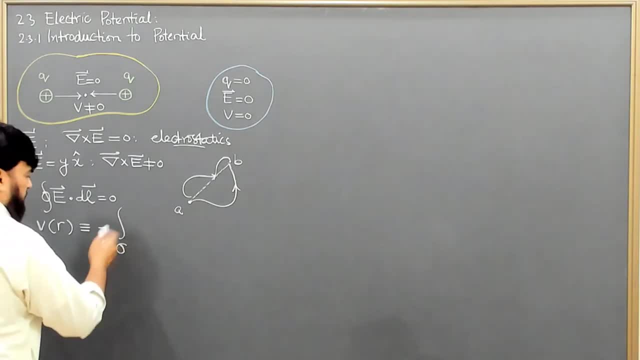 an arbitrary point. O. O is written in this form To R, and this is E dot D L. So this is E dot D L, And now this is. I have. earlier, in the earlier lecture, I have told you that this is actually. 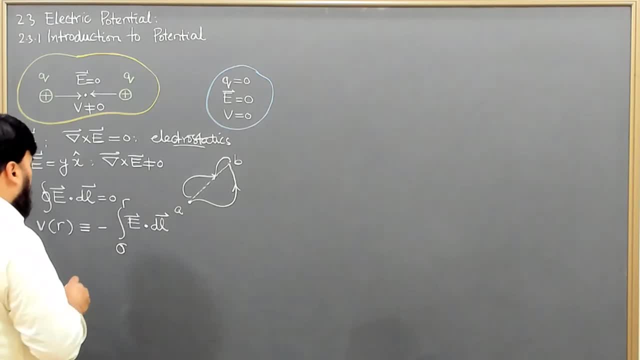 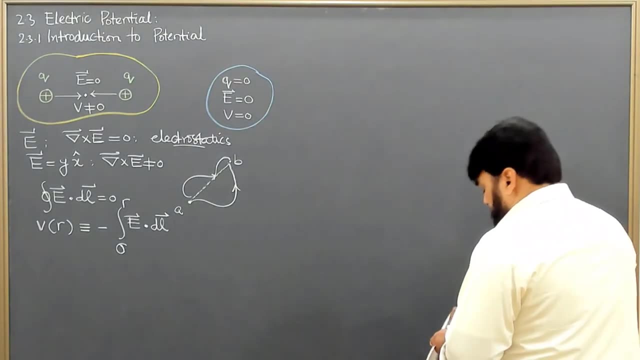 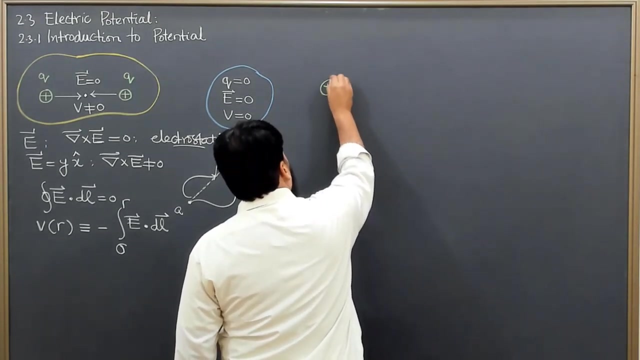 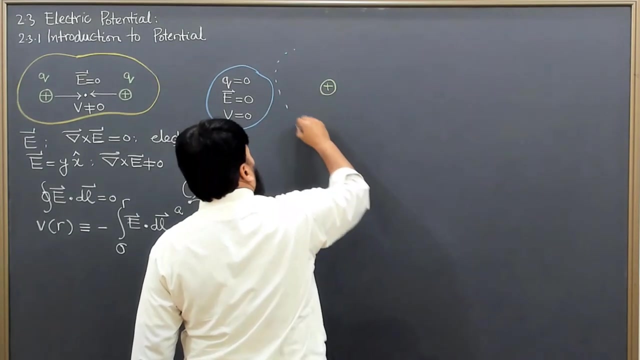 the work done on a unit charge. Now why we are having a minus, Why we are having a minus sign here. I will explain all these things like, for example, we are having a positive charge here And over here, the. this is the vicinity in which this charge is having its impact, and 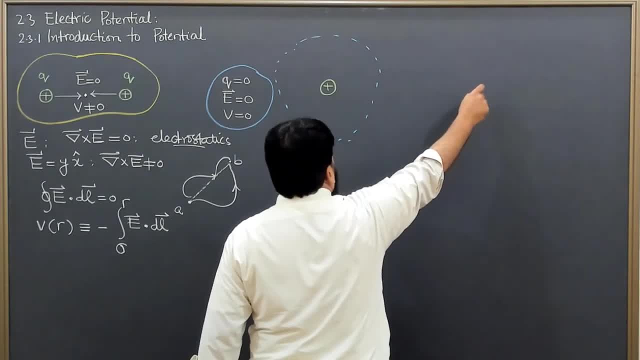 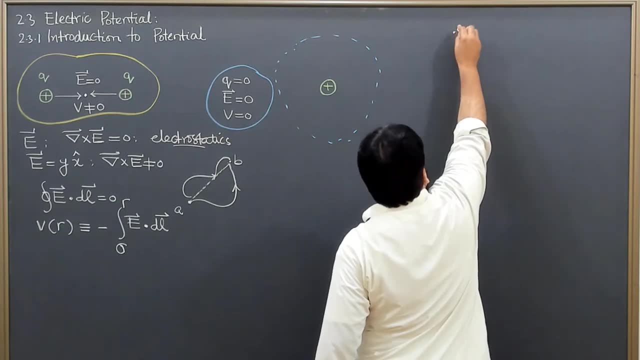 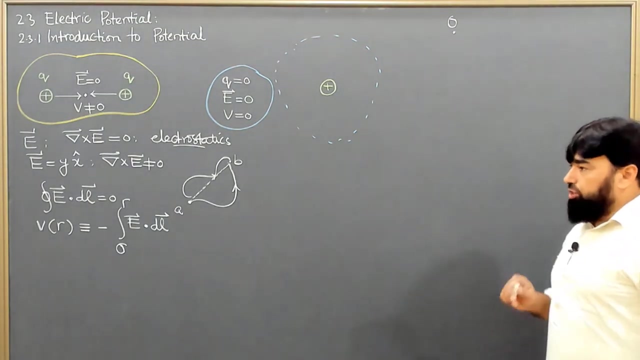 like, the impact is still infinity, And this is the region that I have, This is the region that I have enclosed here And let's say this is our point, which I am calling, is point O, which I am considering it: infinity. Now, keep in mind one thing: infinity never means you move very far. 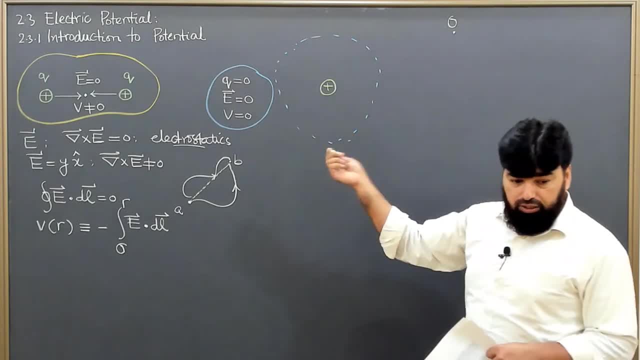 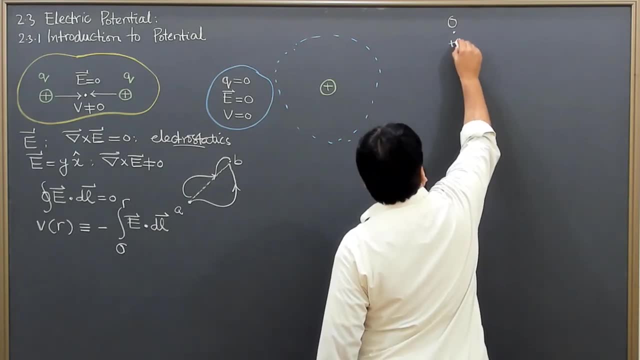 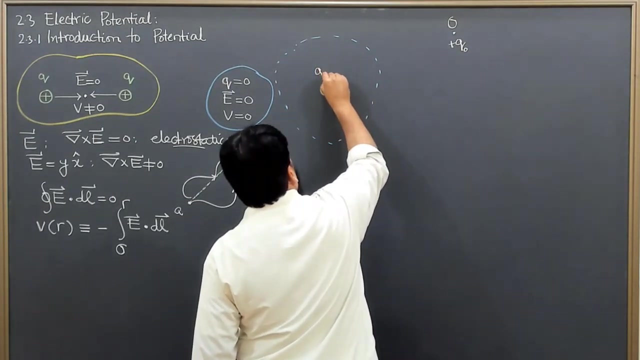 When you go out of the influence of that thing, then it is infinity for it. So let's say this is point O and I'm moving a test charge plus Q here Let's say call this Q, naught, And here I'm having a source charge Q. then when I am moving this charge from this point, 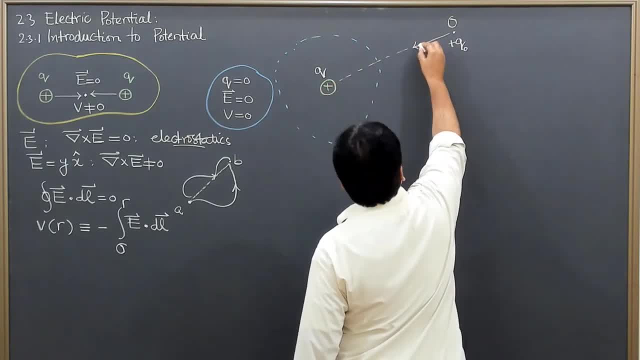 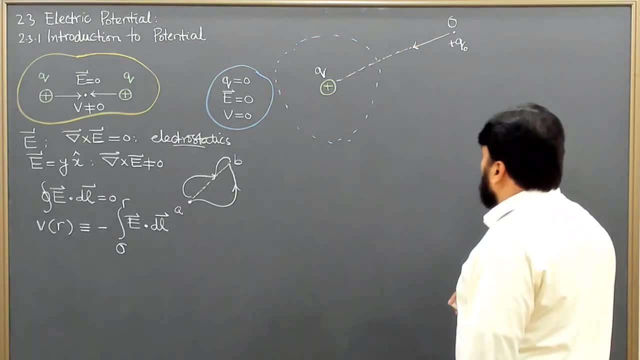 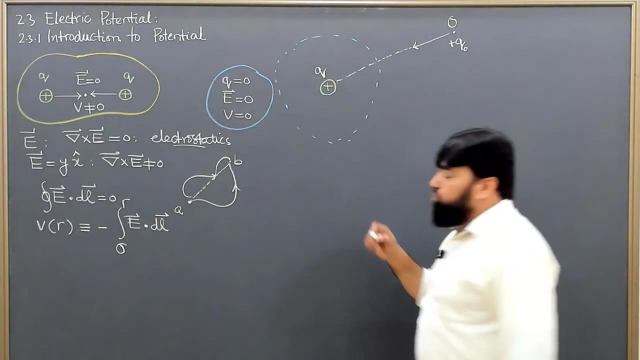 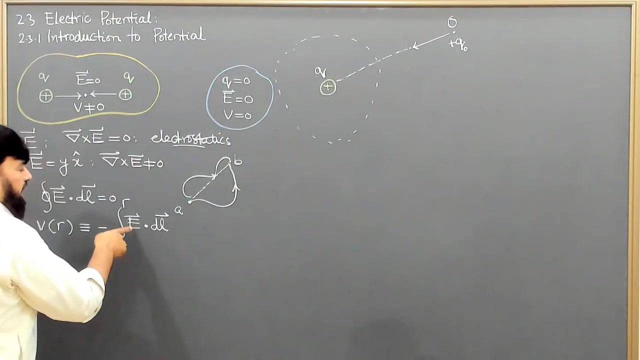 toward this charge. I'm doing some work and that work is converting, that work is being stored is energy in this system. But Think of this thing: I'm coming from infinity towards the charge and I'm doing work against the charge. If I will consider the electric field, then the electric field is doing work in the opposite. 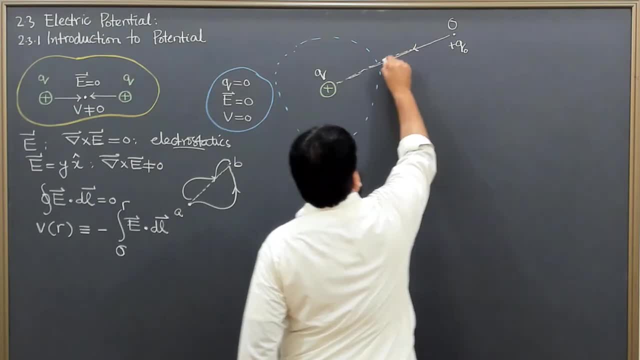 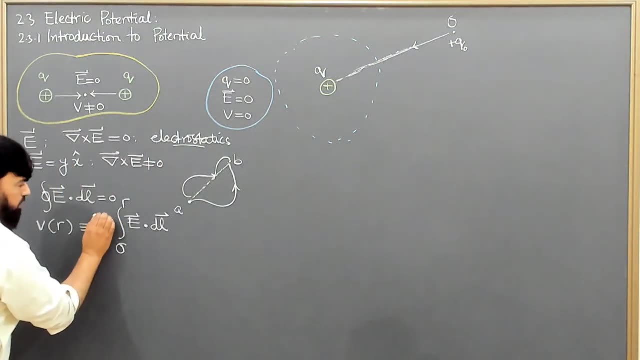 direction is going in the opposite direction and I'm going from there to here, So that's why it is the work of the field. Then it is with plus sign, and the minus sign means that it is the work which is done against this one. 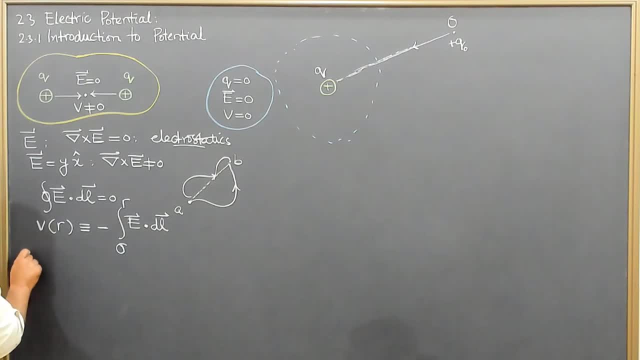 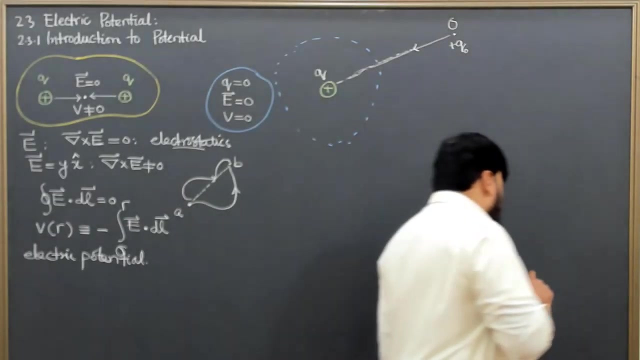 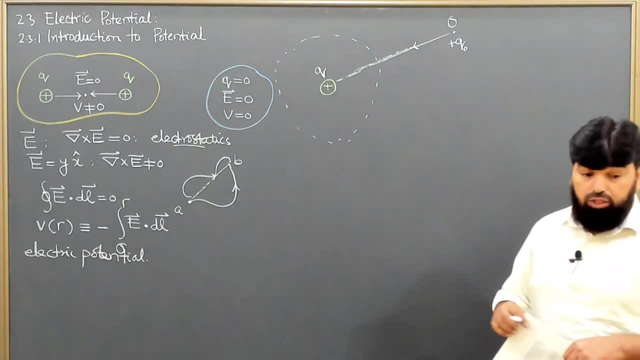 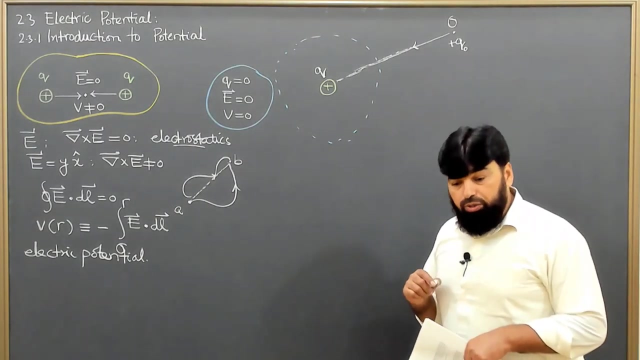 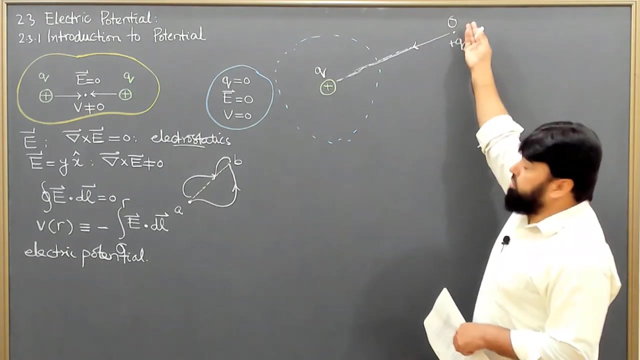 Electric potential are sometime it is called, is absolute electric potential. It is not a physical quantity, because physical quantity means we can measure it, The electric potential we cannot measure. We can measure the potential difference and not the electric potential, because we can't specify what is this point, from, where it is coming in. 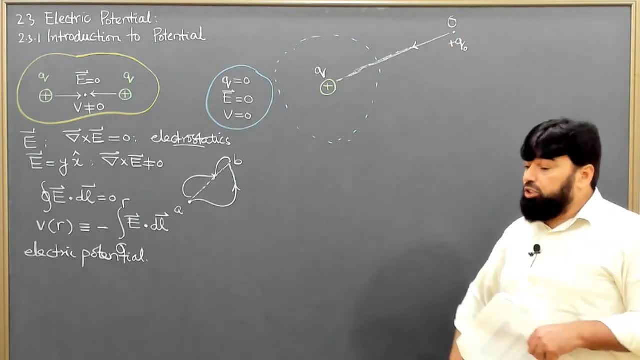 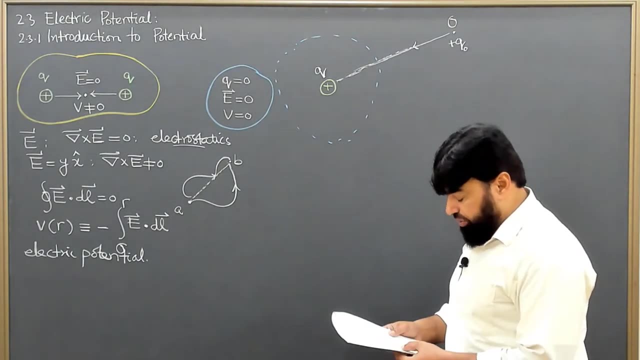 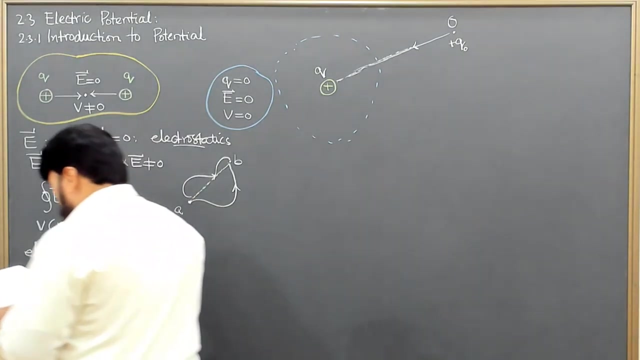 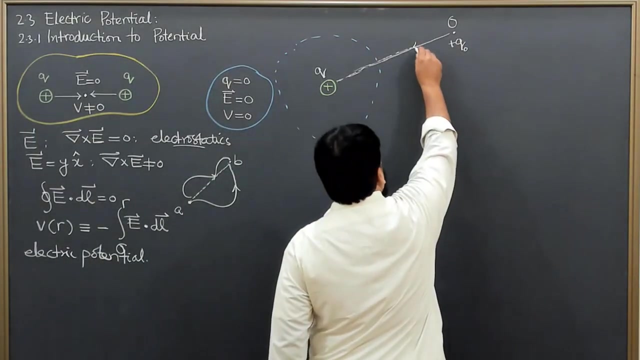 Where this infinity point is. So this is a single value thing and we cannot term it is a measurable thing or a physical quantity. The thing that we can measure is called a potential difference, and the potential difference- Let's say on the way I'm having this is point A. 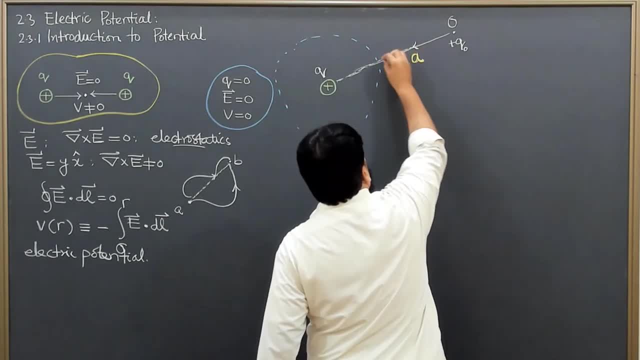 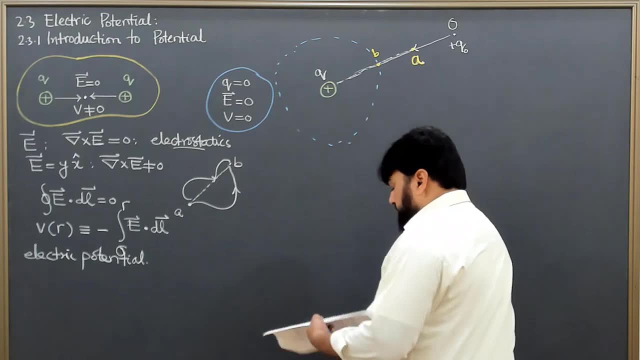 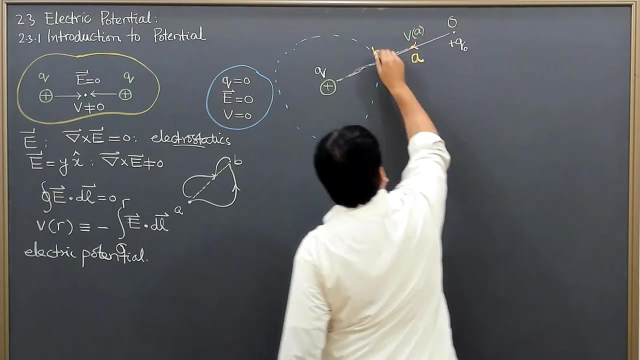 This is point A. This is point A and this is point B. These are the two points And now I know that the potential, the value of the electric potential at V It a point is V A and the value of electric potential at this point is V B. 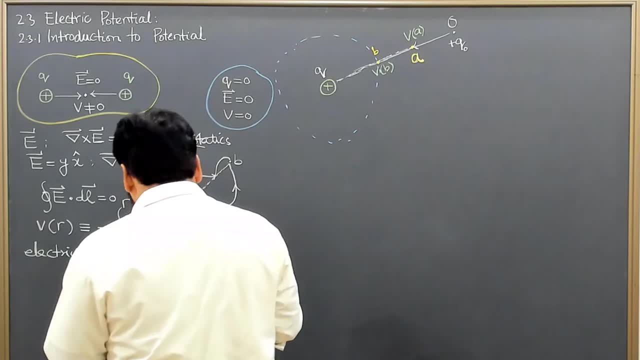 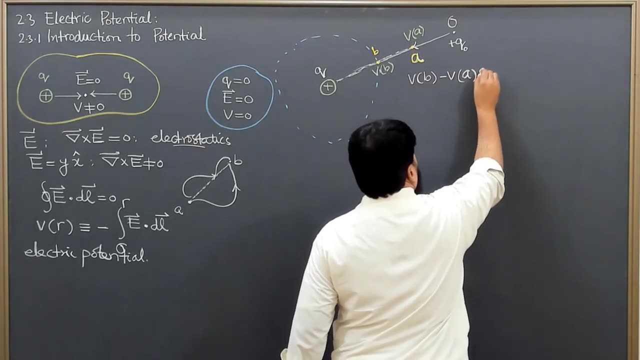 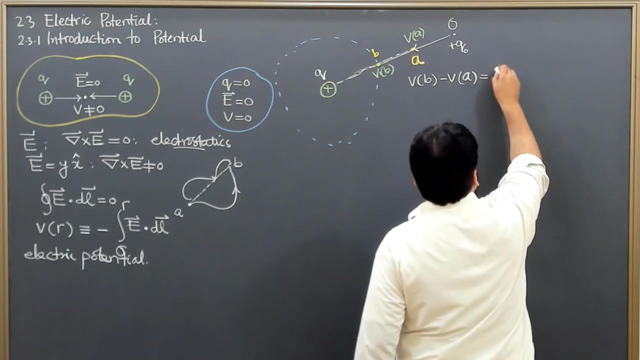 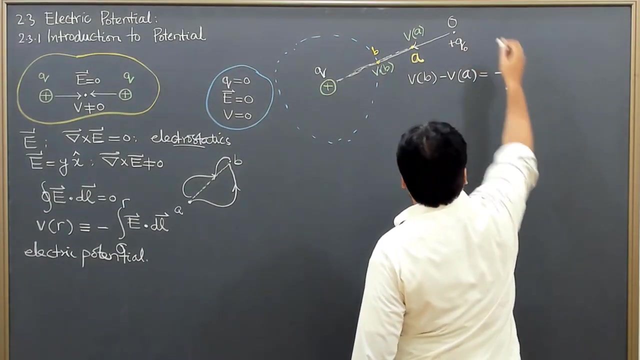 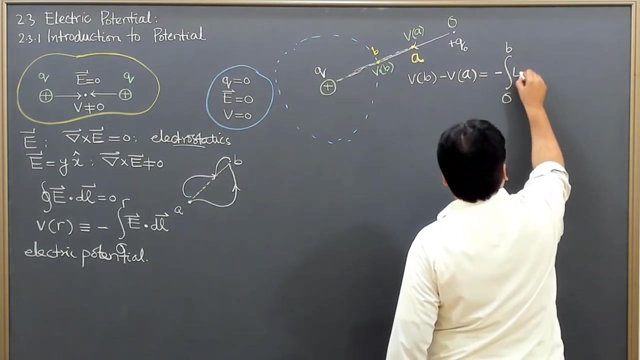 And then I can write that V B V B minus V A is equal to Now. I can write here that minus Now V B V B means from this infinity point O I will reach the B point, and then this is E dot D L. 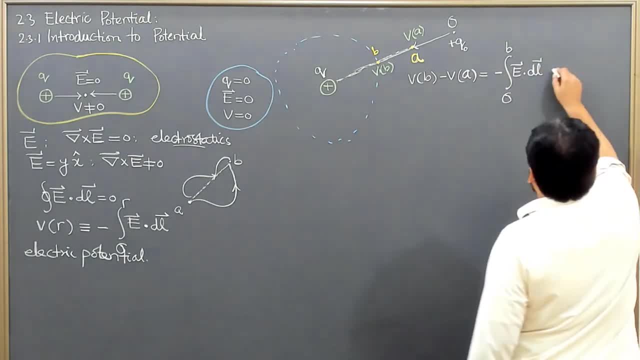 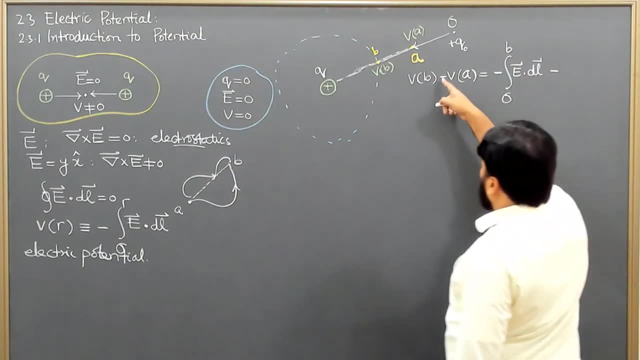 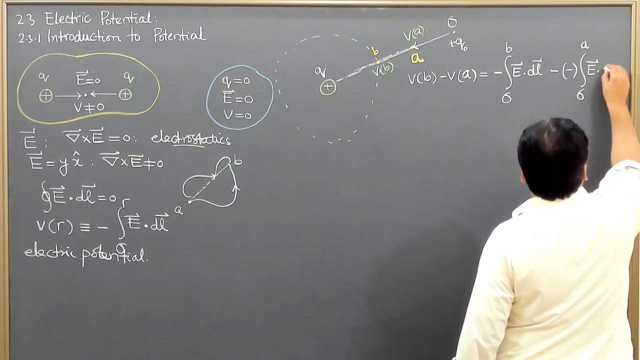 And then minus here and another. minus means this minus, It is this one. And then what is V? A? V? A is again with minus sign, and then integral from point O to point A, And this is E, dot, D, L, Like when moving from here. 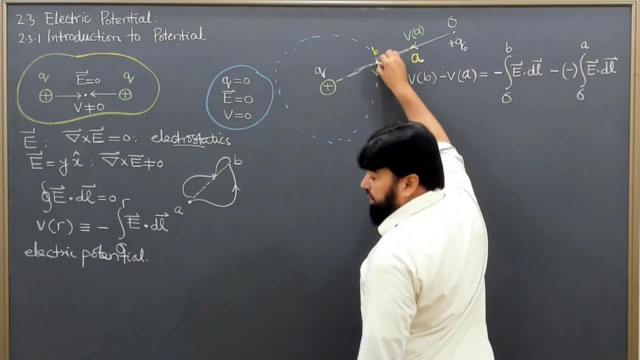 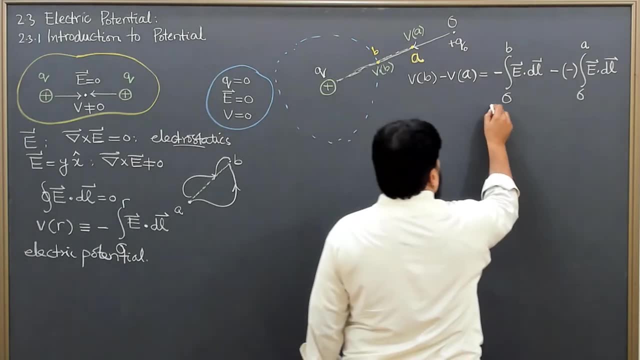 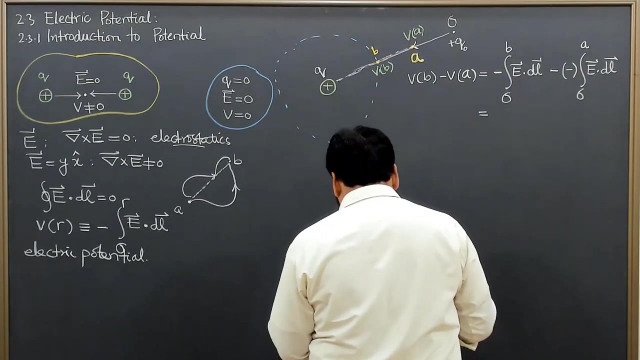 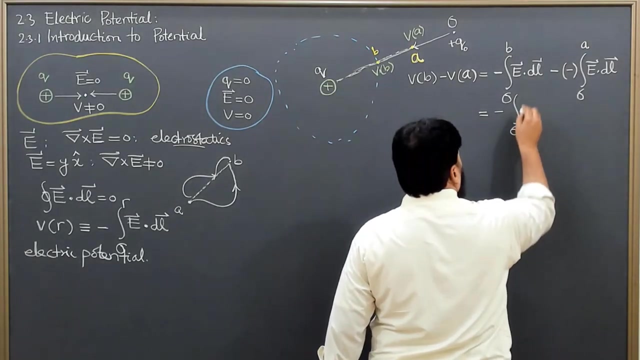 I am going independently to point B And then from point O to point A and it will be equal to this And this thing- I can write that this is equal to This- will become plus, and I can write: this one Is minus. integral from O to B. 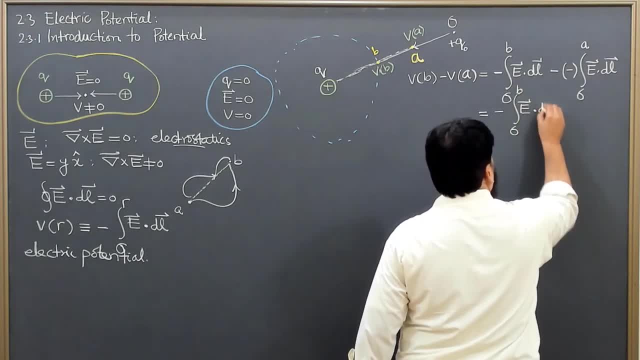 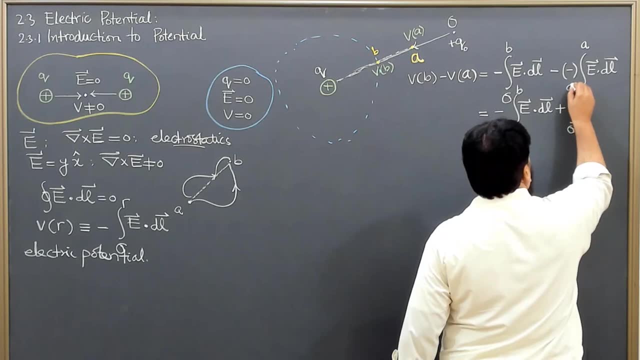 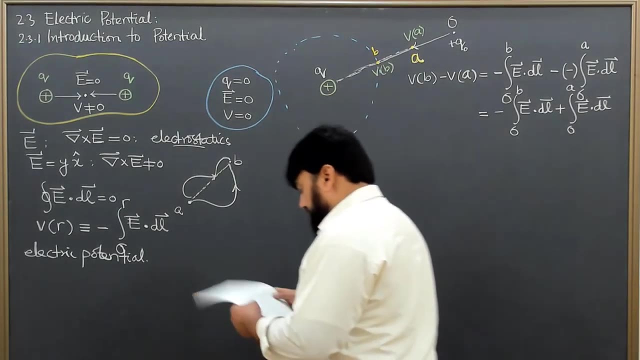 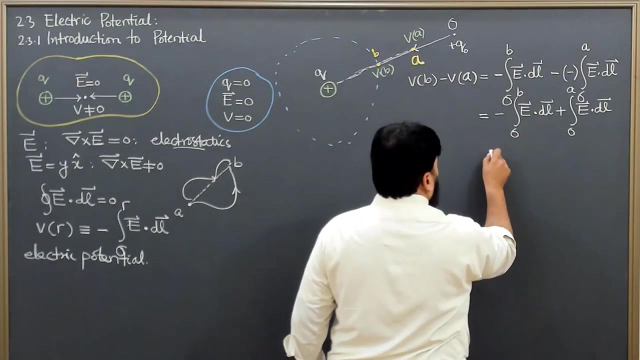 E dot D L, Plus integral from O to A point: E dot D L. Now, what about here? This thing I can combine now, Like I can write that this is equal, This thing is equal to, I can combine and I can write: 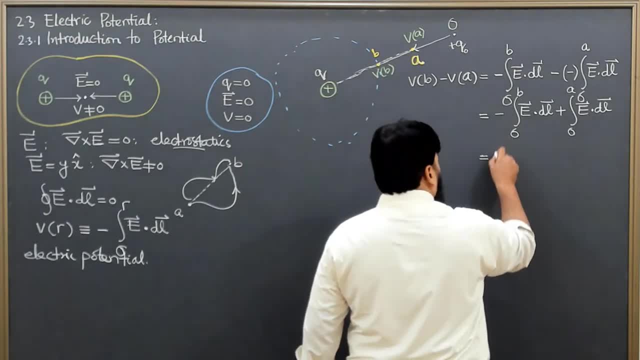 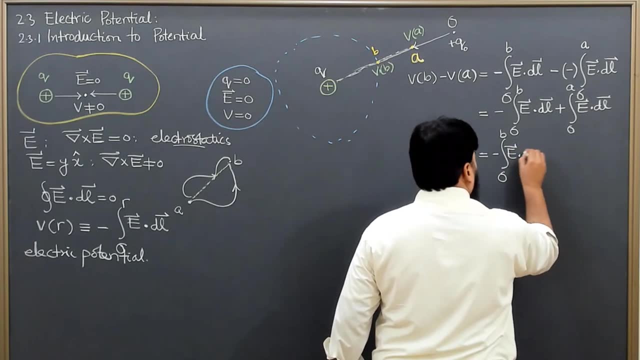 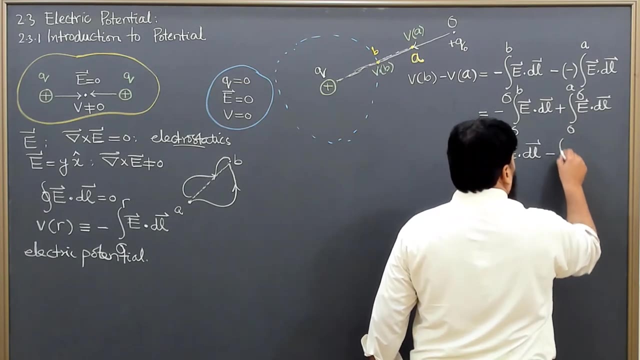 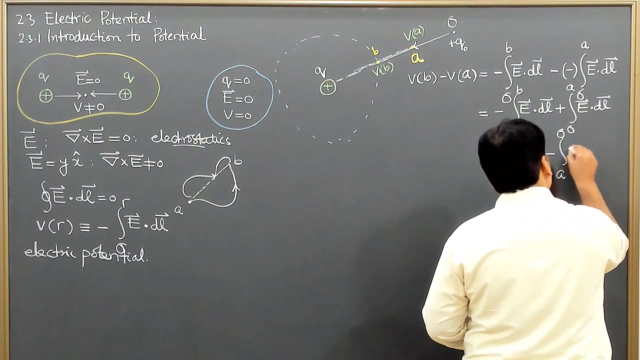 This is from Minus, from point O to point B, E dot D, L, And if I reverse these two points Then minus sign will occur. And this is from point A to O And E dot D, L, And reversing the limits of the integral will be equal to this. 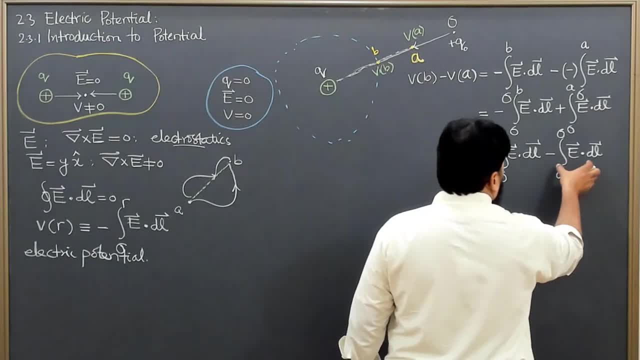 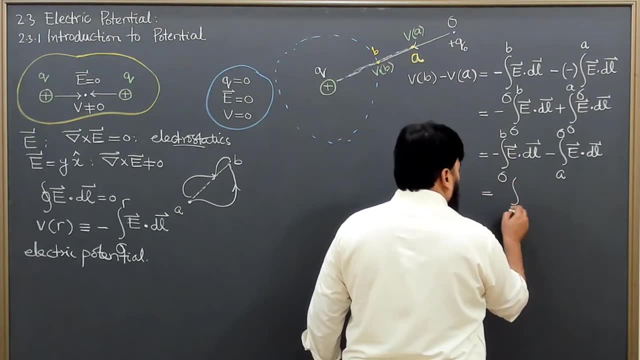 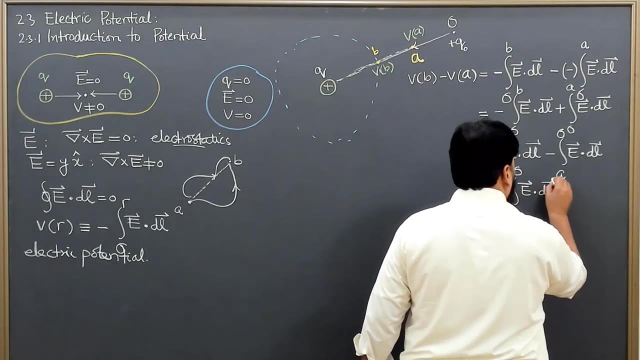 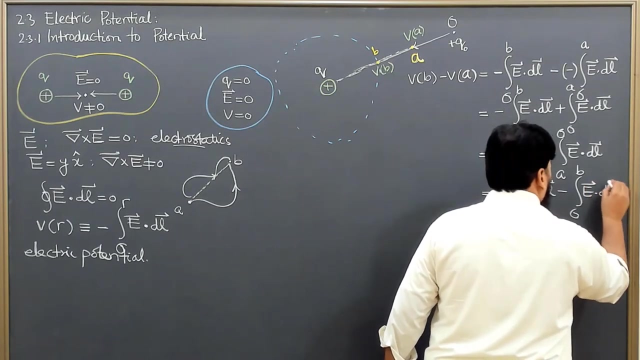 And now I can write. If I write this one earlier And this one later, Then this is equal To minus A to O And E dot D L, Minus O to B And E dot D L, And this thing simply is equal to minus. 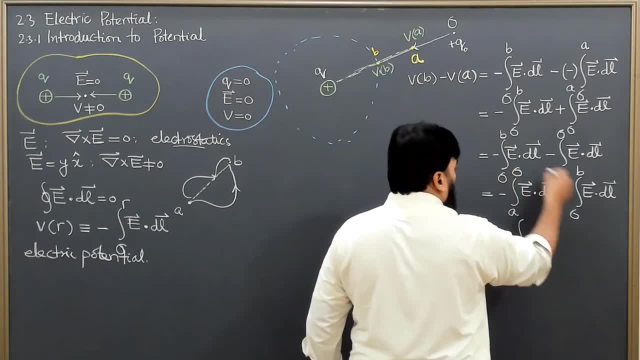 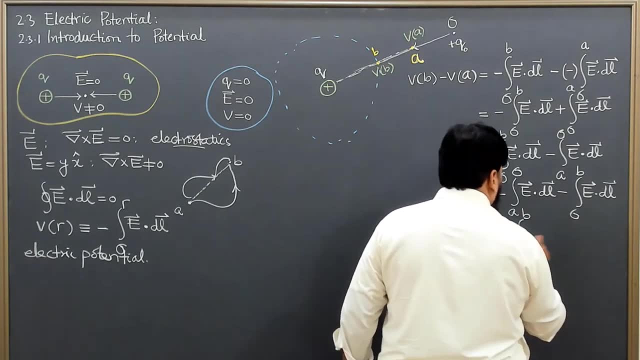 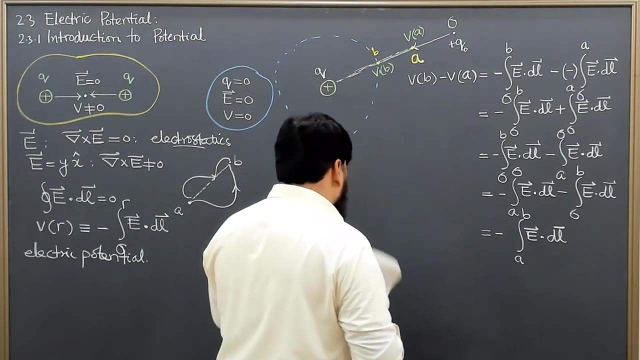 Now from A to O and from O to B. So this I can write from A to B in a combined form, And E, dot, D, L. So this is this side that I can write. Now, what about this side? We know that. 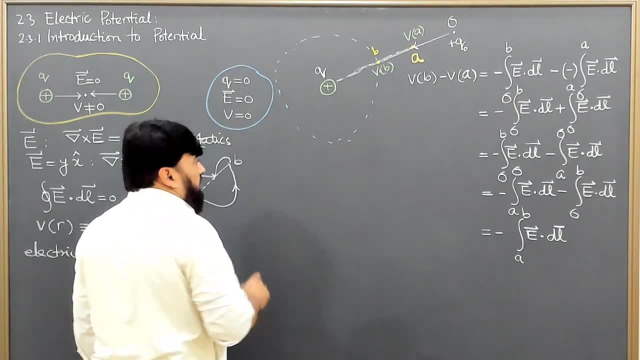 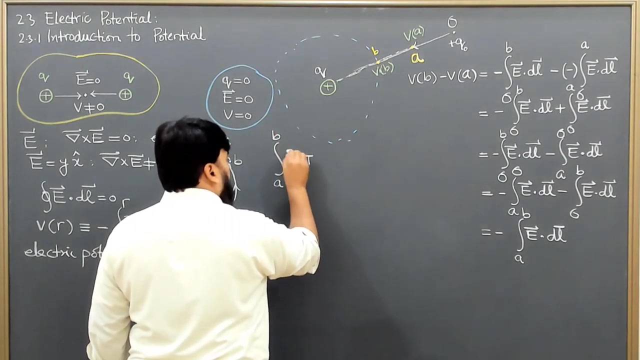 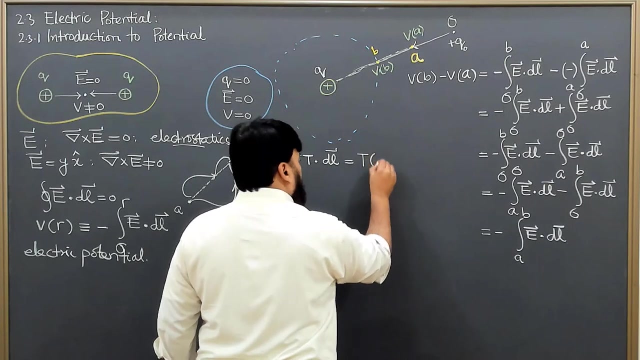 What is V B minus V A? The Theorem of The fundamental, theorem of gradient. We have said this thing: That integral From A to B Gradient of T, Dot, D, L Is equal To the value of T in the end points. 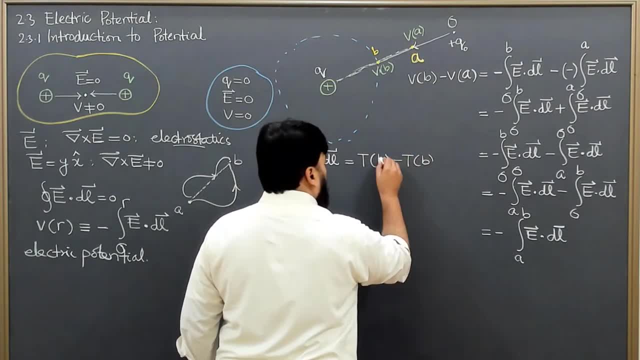 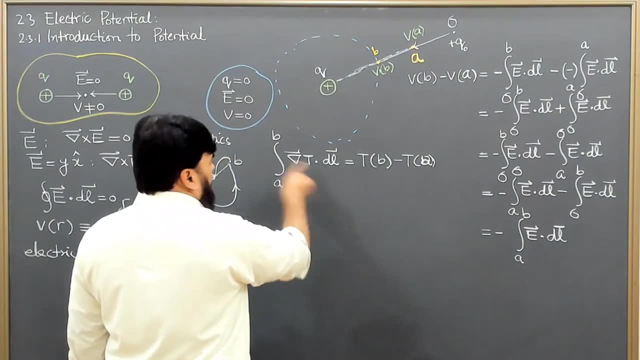 T A minus T B, T B minus T A here. So this is the The value of This gradient: T dot D, L. So incorporating this result. This is the fundamental theorem of Gradient, So we will incorporate This result here. 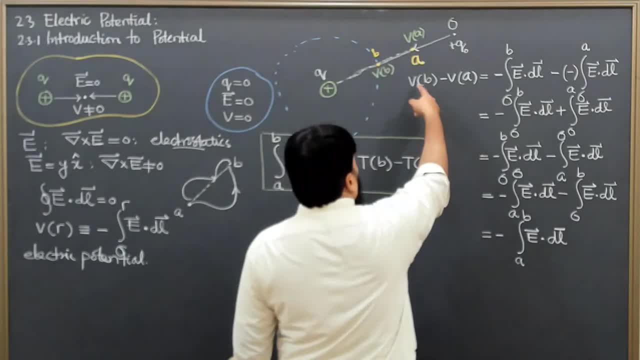 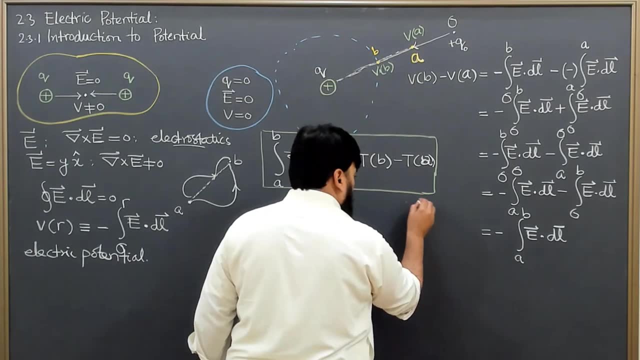 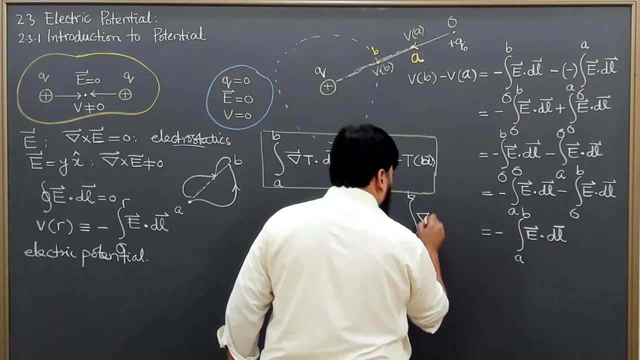 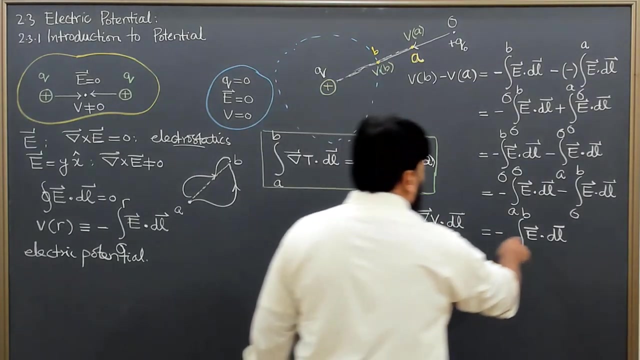 And this is giving us. I can write For V T here. So it means That this thing is equal To: From A To B And gradient Of V Dot D, L. This is equal To minus. 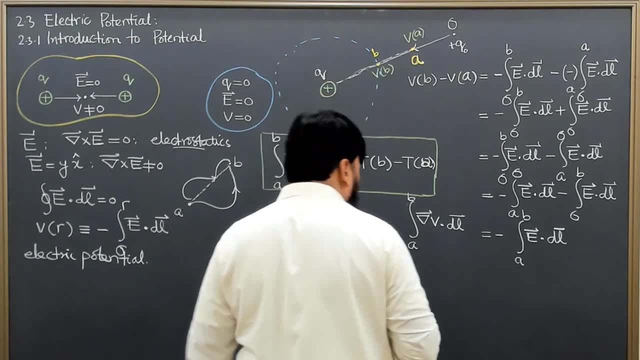 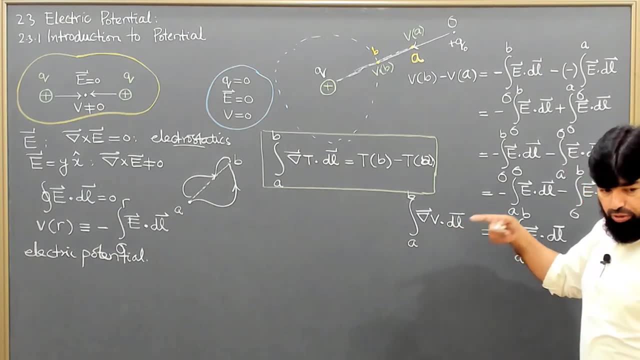 E Dot D L. And now from here, The end points are the same And it's a frictional length, The smallest, The minimum Length possible, And this is E dot D L. So the same limits, Same length. 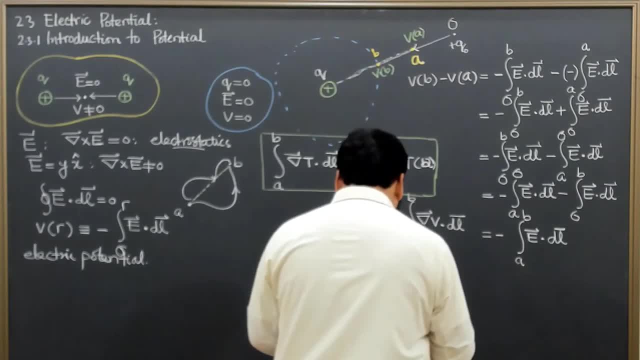 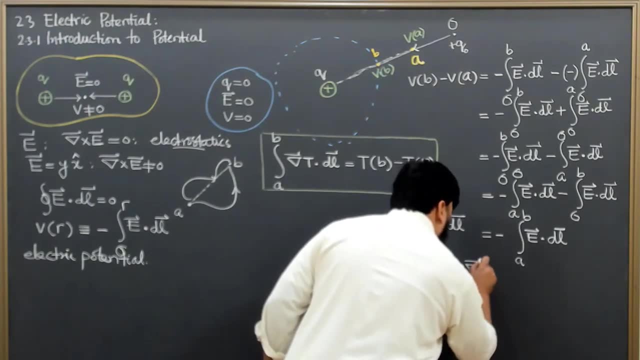 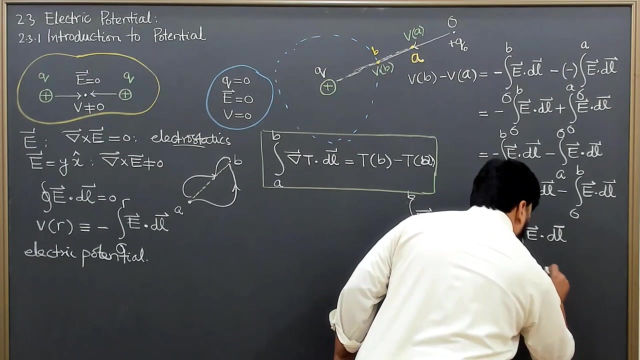 Element. So the Integrant Will cancel out Here And I can Simply write From here That Gradient Of V Is equal To minus E, Or this I can write Is: E equals. 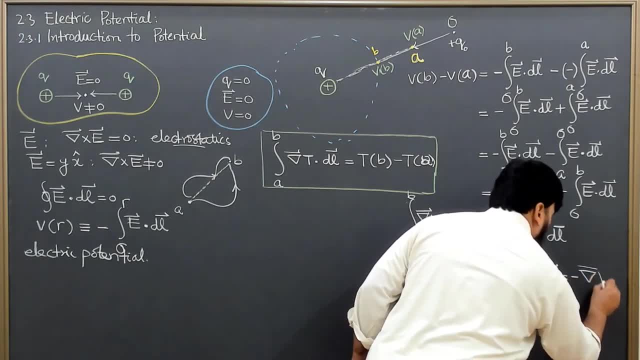 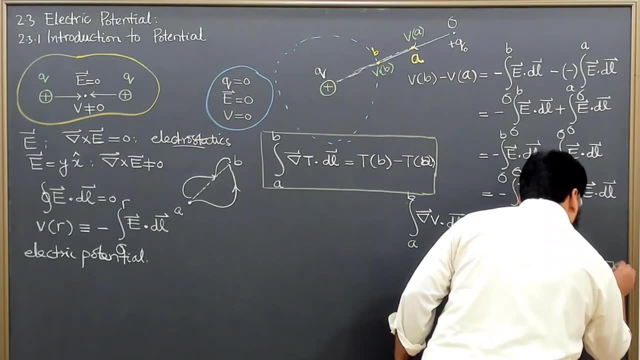 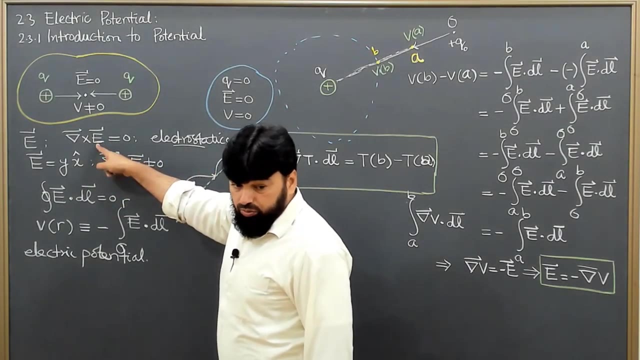 Minus Gradient Of V, And this is the result. We were behind That. When The curl Of E Is equal To zero Means The lines Are not Curling, They are going. 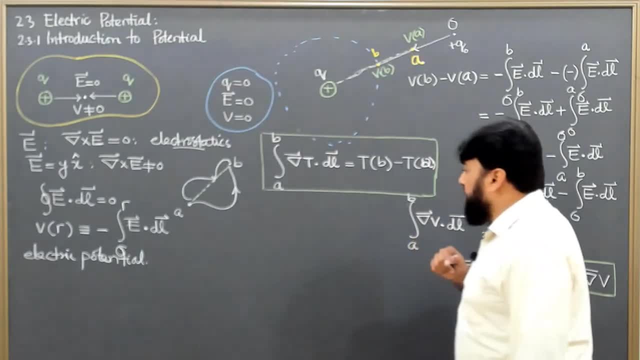 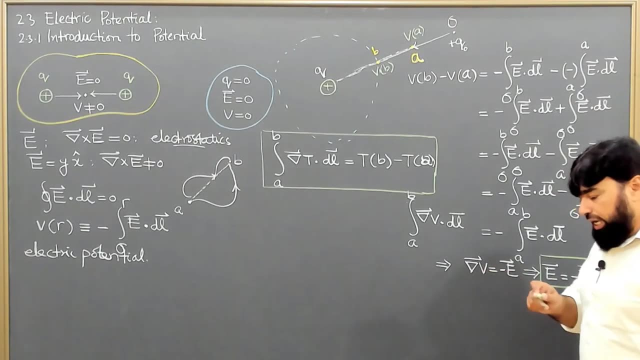 Straight, And when They are going Straight, It means They are diverging. When They are diverging, Then They are going In straight Line, They are not Curling At all. It means That. 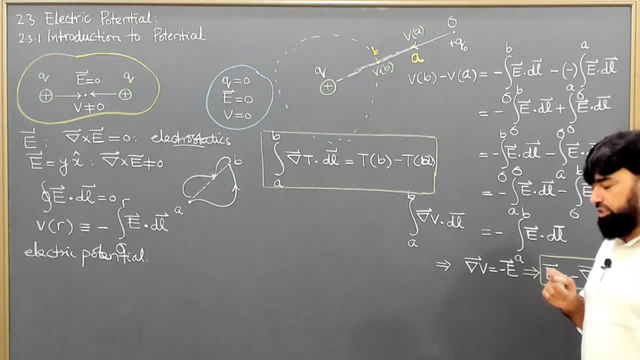 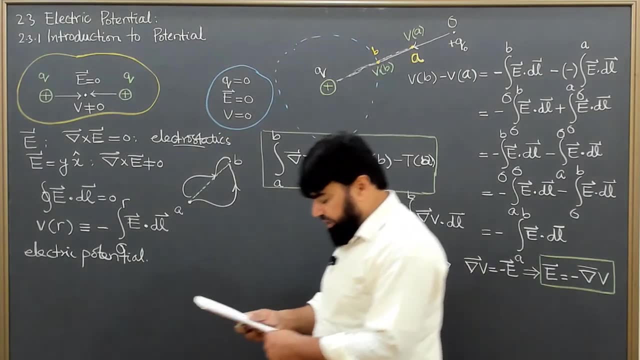 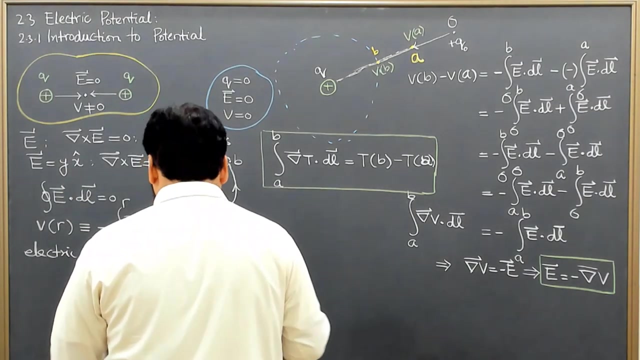 Electric Field Is The Maximum Change In A Given Direction And I Can Write That Electric Field Is The Negative Gradient Of Electric Potential. So These 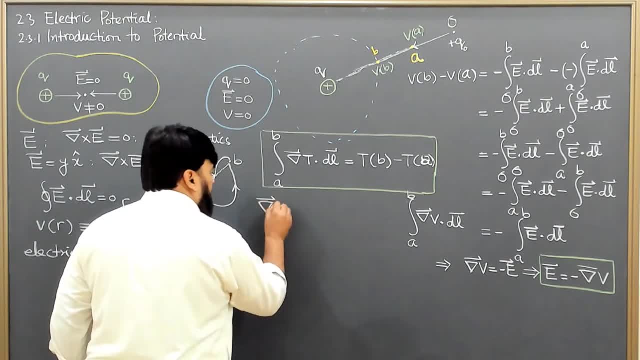 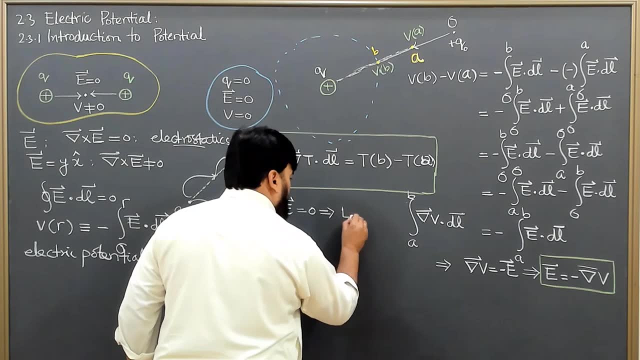 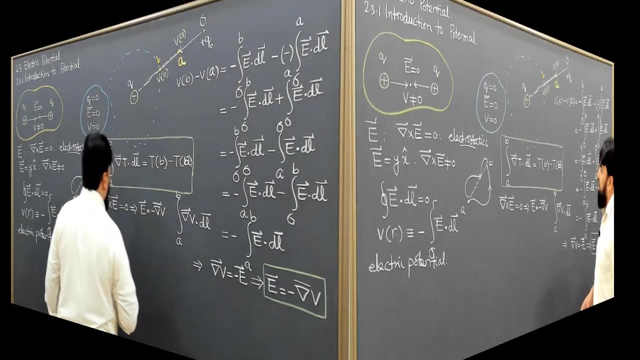 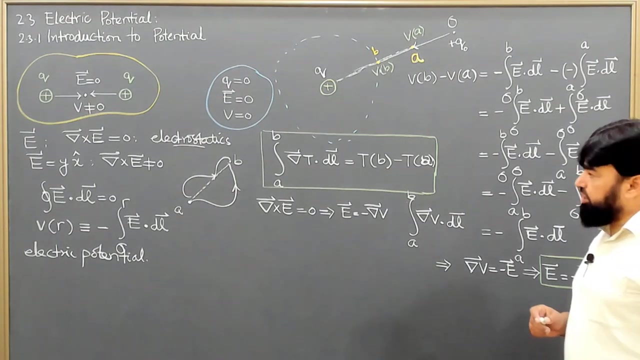 Two Things I Can Now Summarize. To Zero Implies That E Is Minus Gradient Of V. Now Some Comments On The Electric Potential, The 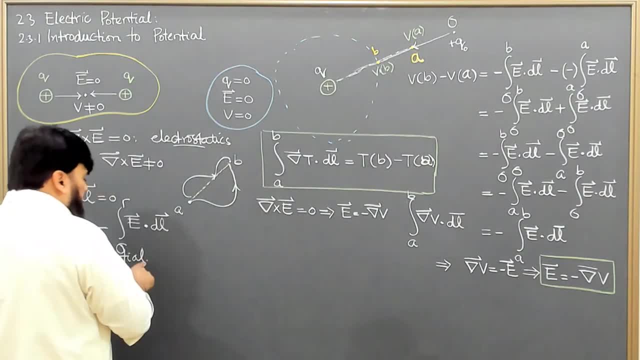 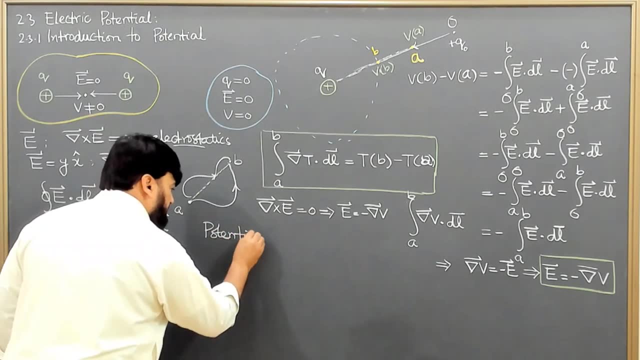 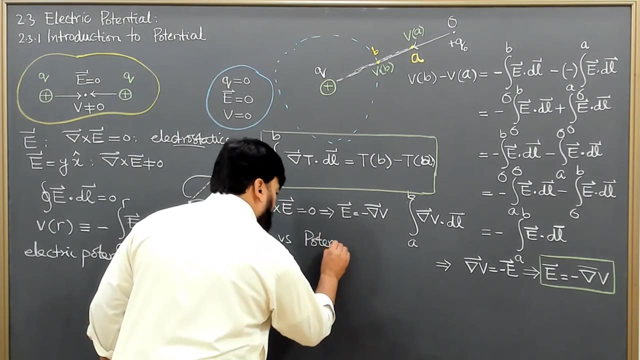 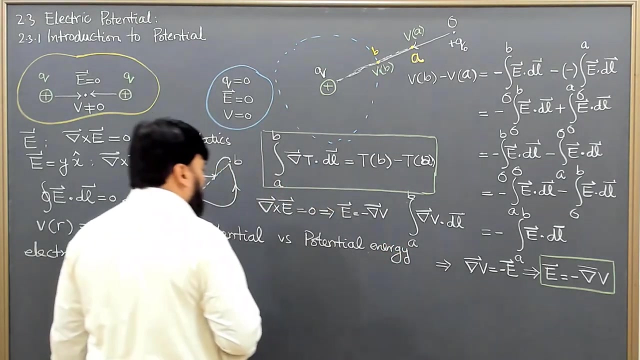 Very First Thing. The Very First Thing Is That Versus The Potential Energy, Are These Two The Same Thing, So They Are Completely Different Things. 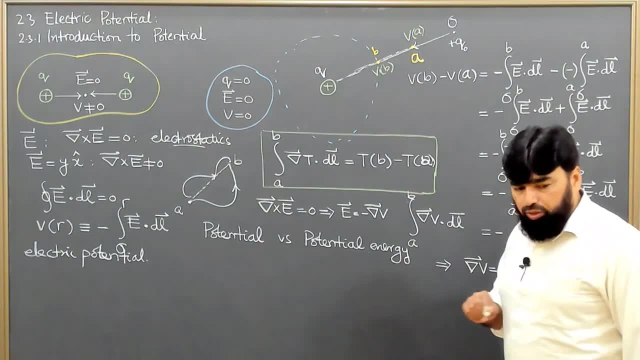 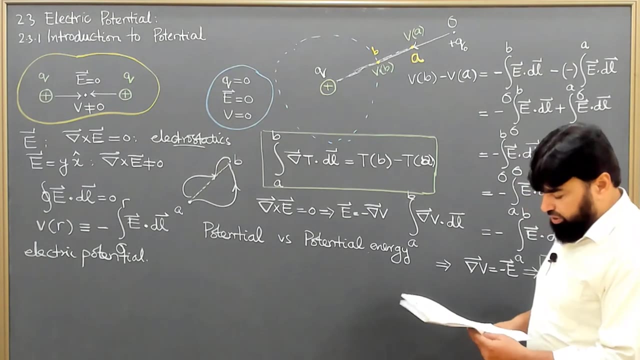 They Are Not. The Same Electric Potential Has Nothing To Do With Each, So Dimensionally They Are Different Things, Although Their Names Resembles. But 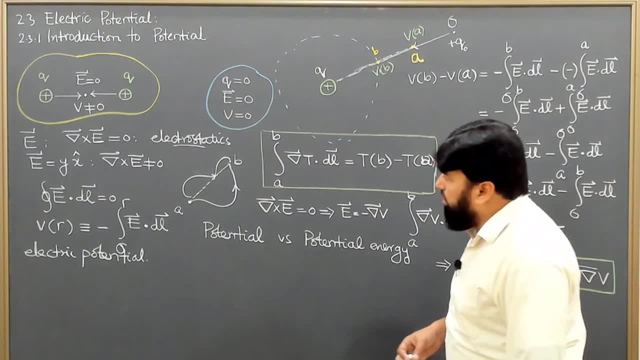 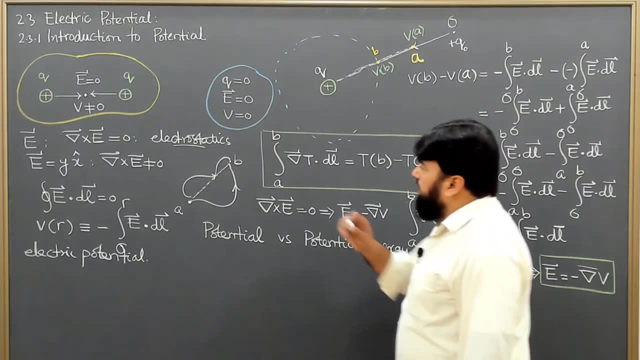 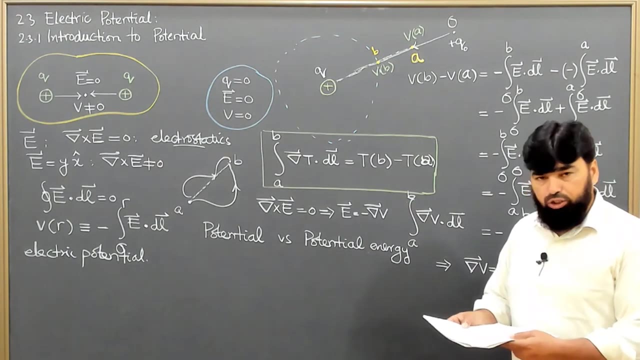 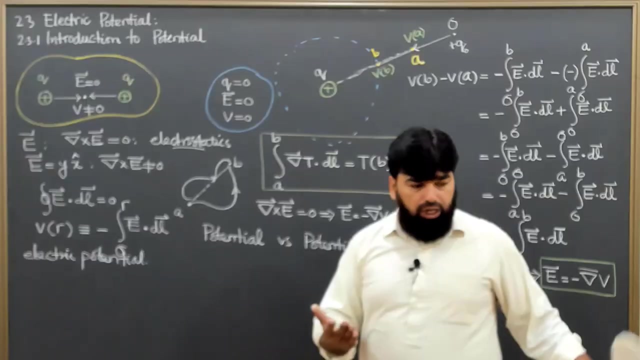 They Are Completely Different Thing. I Have Earlier Discussed That The Advantage Of Going To Electric Potential Is Home, So If I Will Be Having 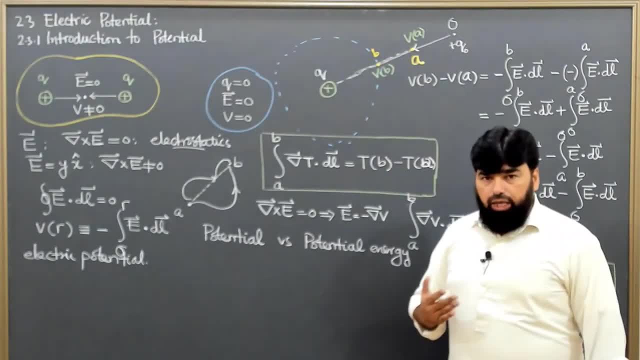 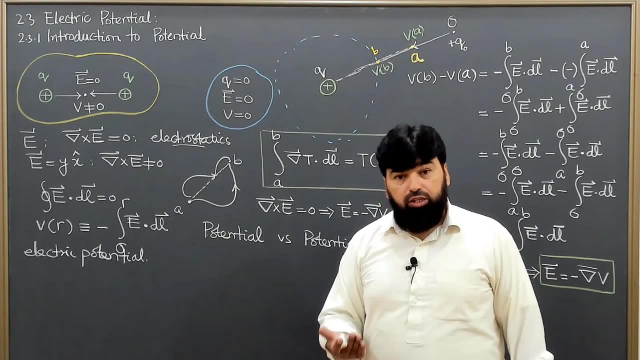 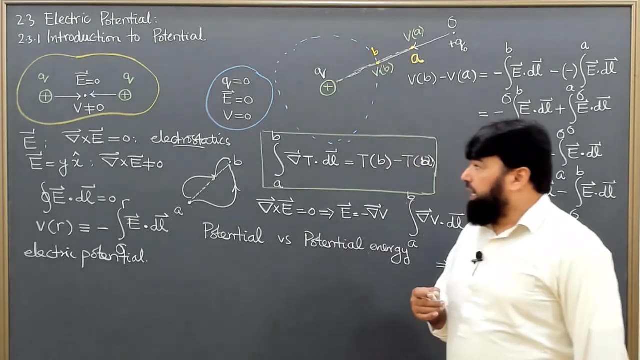 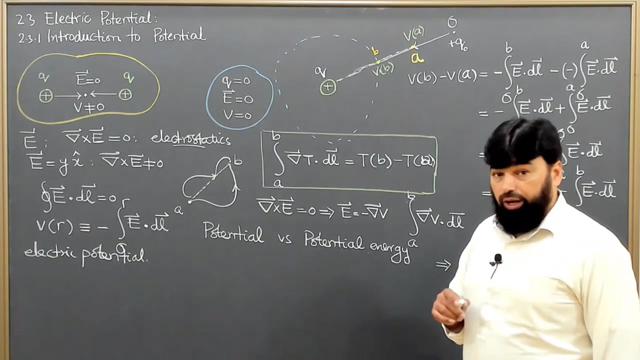 That Meter And There Are, For Example, Charges On One Wall, In On The Other Wall, And I'm Checking Through The Meter. This Conclusion Will: 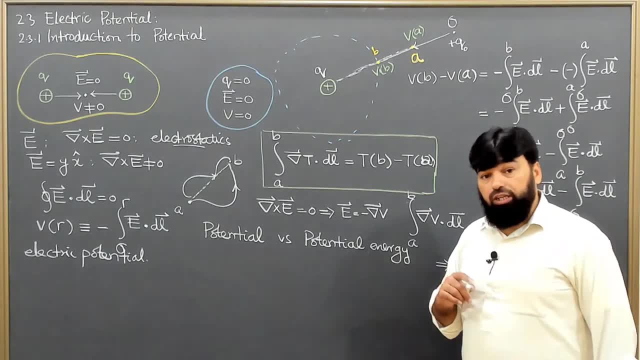 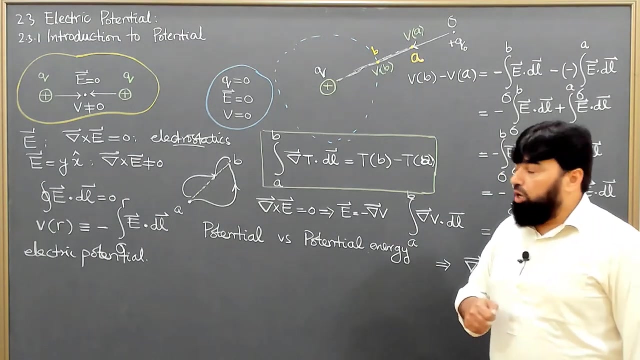 Not Be Correct Because I Will Have To Keep In Mind The Victorian Nature Of The Electric Field. My Meter Should Have Also Another Option To 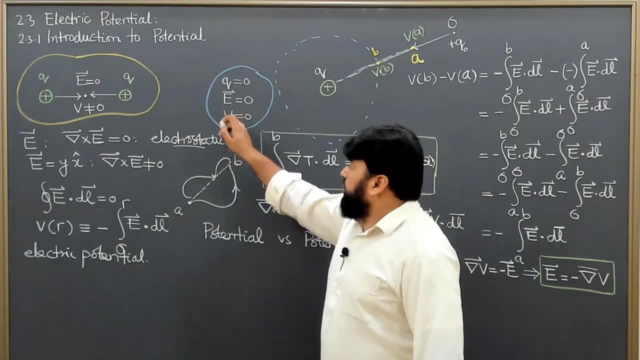 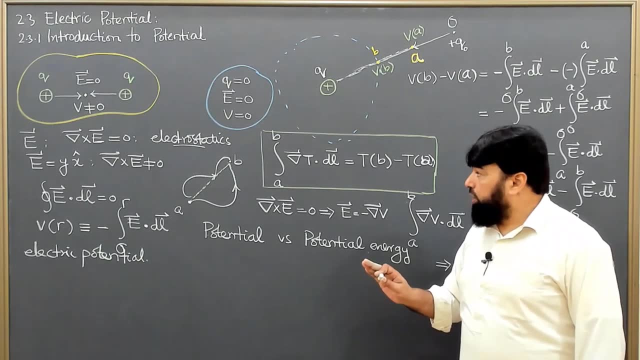 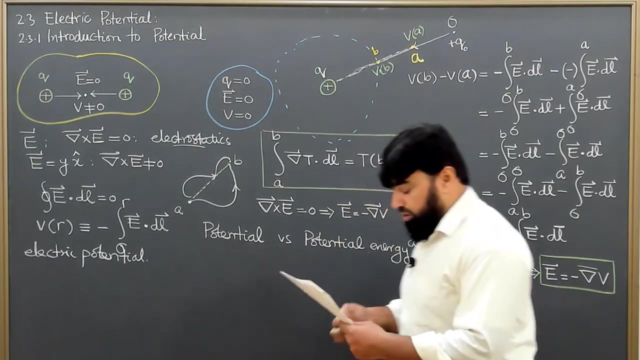 Our Charges, And If The Potential Also Come Out To Be Zero, Then I Can Very Quickly Say That There Are No Charges Here In This. 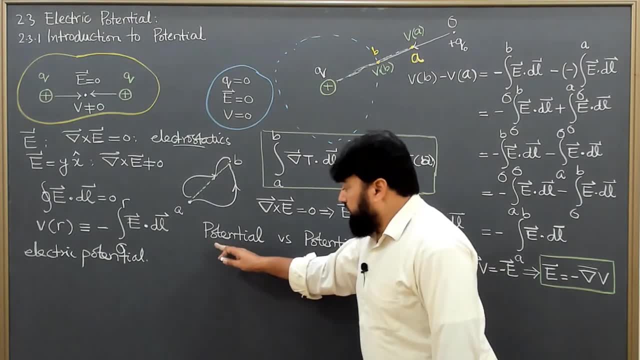 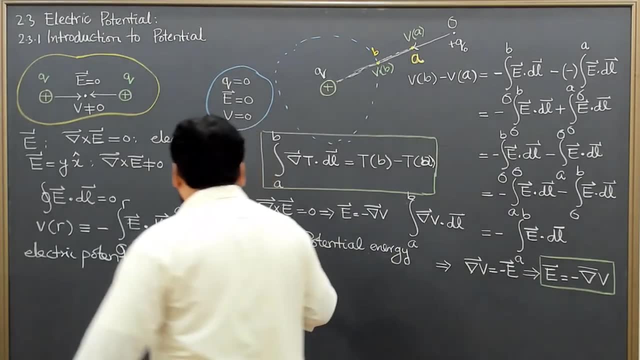 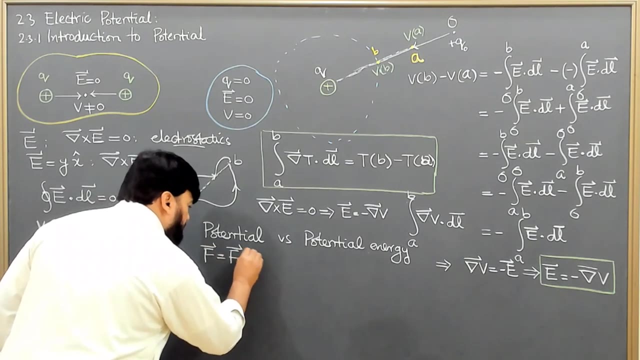 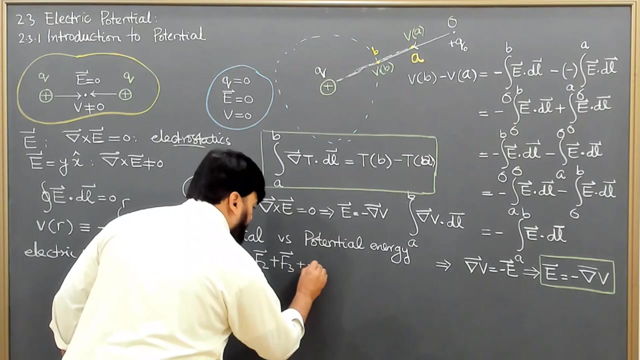 Room. So I Show Of Being The Superposition Principle. So Yes, Electric Field. Just Like When We Write Forces, Electric Forces, It Is Being The 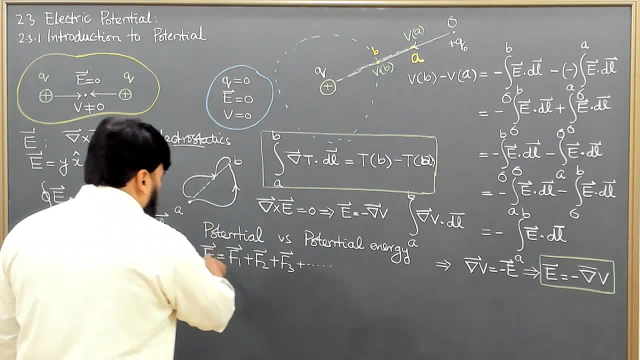 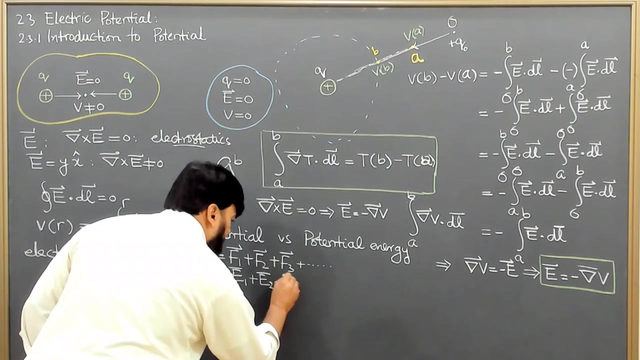 Superposition Principle, Like Many Charges Here. So The Electric Field, Which Is The Force Per Unit Charge. This Is Also, This Is Also Being The 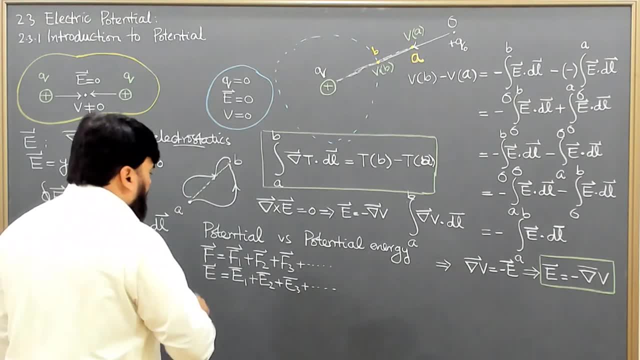 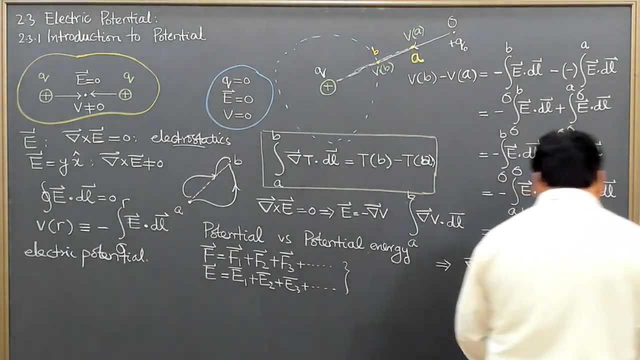 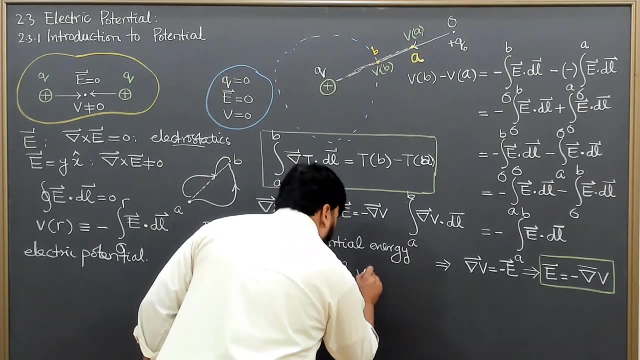 Superposition Principle: E1. Plus E2. Plus E3. And So On. Now, These Are The Superposition Principle. So Yes, It Is Also Being The 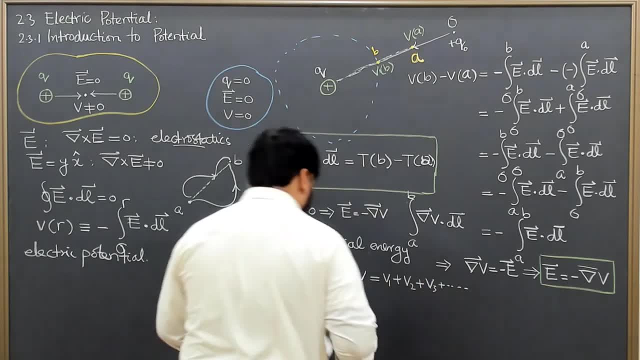 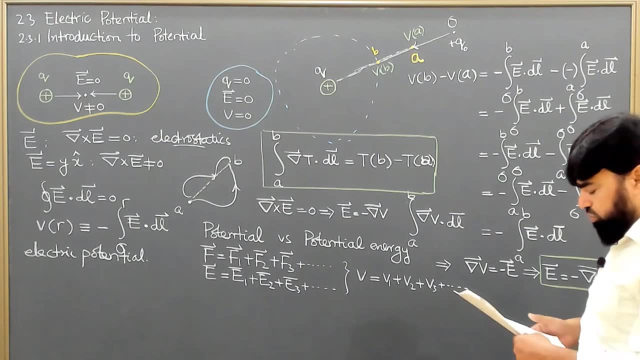 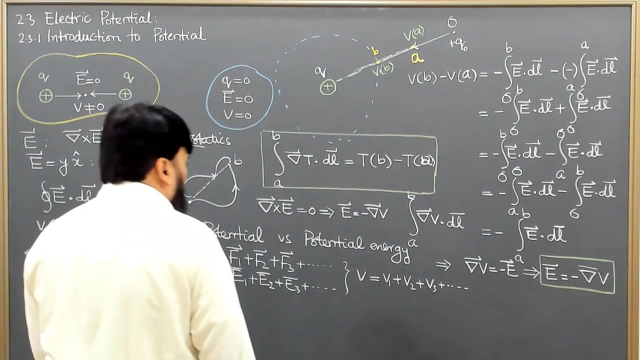 Superposition Principle V Equals V1. Plus V2. Plus V3. And So On. So The Potential, The You Are, The, I Can Say That From. 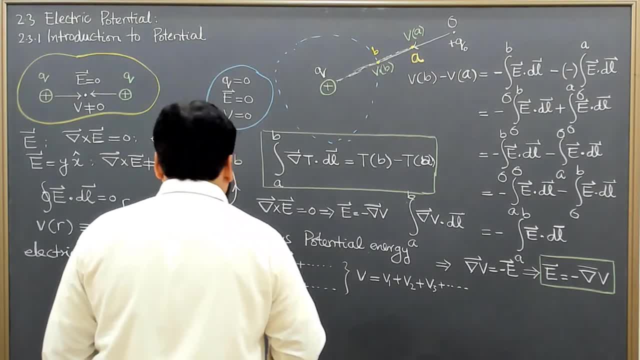 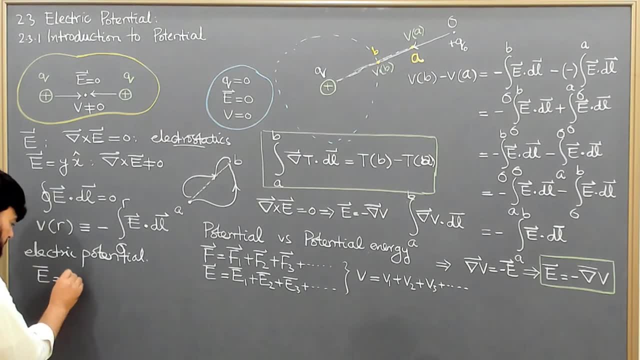 Here. From Here I Can Write This Thing In More Simpler Form: That E Is Equal To Minus Gradient Of V, Then The Minus. 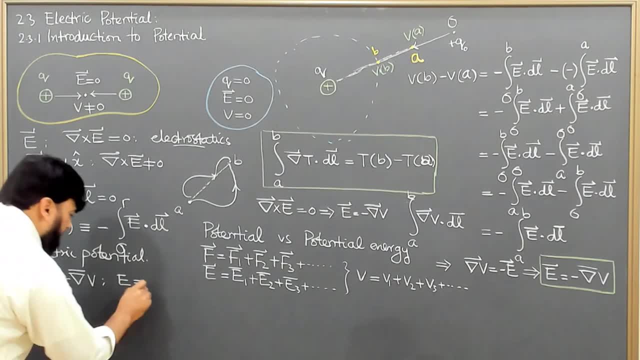 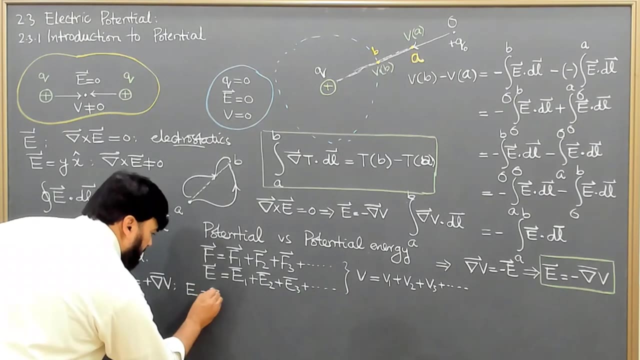 I Can Write In Magnitude Form Here This One Minus- Sorry, With No Minus Sign- Gradient Of: We Are In One, In One Dimension.